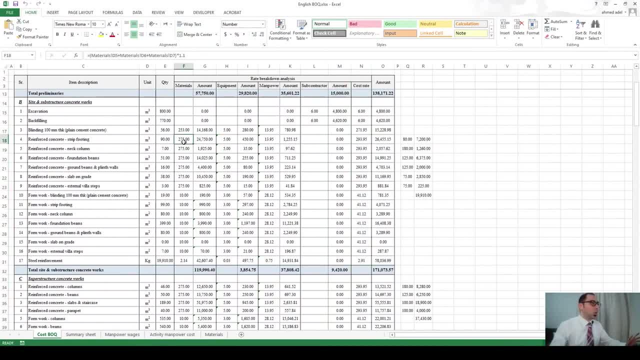 rates has a breakdown How much the material will cost, how much the equipment will cost and how much the manpower will cost, And if there is any subcontractor included in the same item, how much the subcontractor will cost. So, material plus equipment plus, manpower plus. 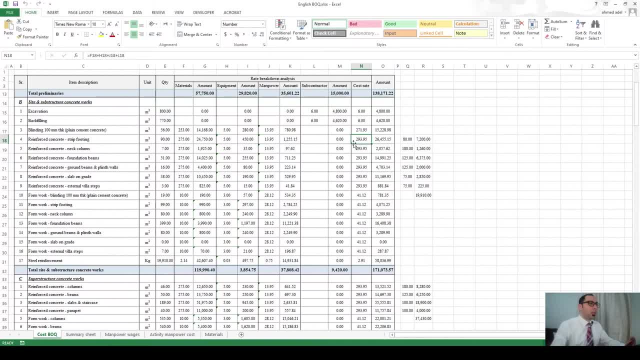 subcontractor will give us the cost rate, And cost rate means how much this item will cost me in order to do it. And when we speak about cost guys, there is more than one type of cost estimation or cost methodologies, Like there are conceptual cost estimation methodologies and there is 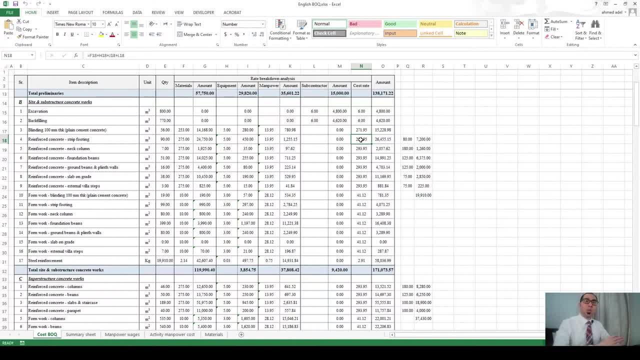 something called deterministic or definitive cost estimation. And what is the difference? Conceptual cost estimation is that when you refer to some historical data in order to estimate a new project. But it is not accurate, guys, It is just something conceptual. For example, there is some method called the end. 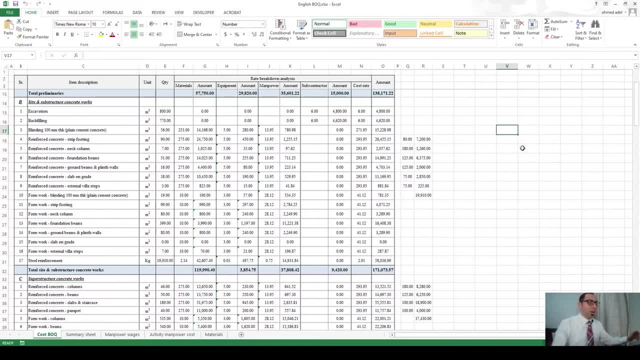 unit method. And what does that mean? For example, if I executed a hotel that has 1000 rooms at the cost of 100 million, let's say So, 100 million. So now a hotel that had 1000 rooms will cost 100 million. So how much is the? 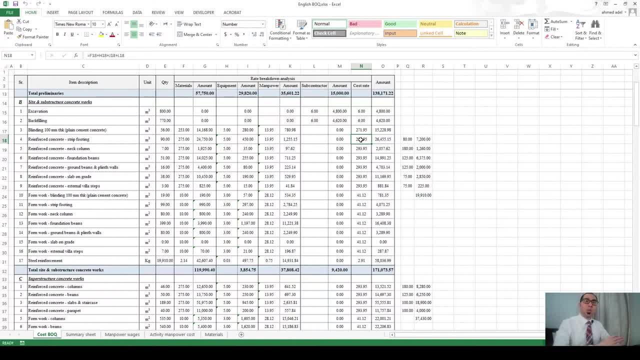 something called deterministic or definitive cost estimation. And what is the difference? Conceptual cost estimation is that when you refer to some historical data in order to estimate a new project. But it is not accurate, guys, It is just something conceptual. For example, there is some method called the end. 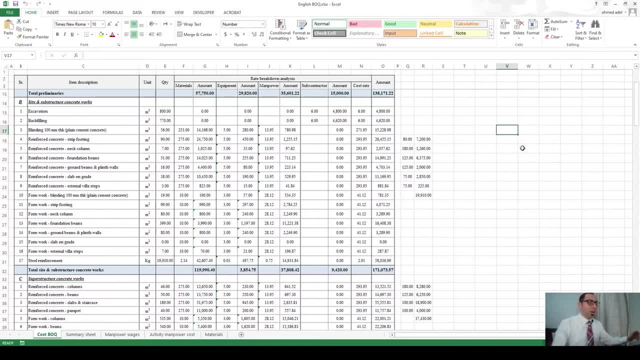 unit method. And what does that mean? For example, if I executed a hotel that has 1000 rooms at the cost of 100 million, let's say So, 100 million. So now a hotel that had 1000 rooms will cost 100 million. So how much is the? 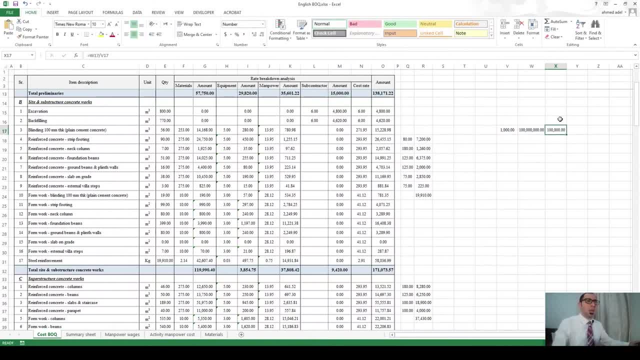 cost per one room. This divided by this, The room will be about 100,000.. So what if I have a new hotel that has 1500 rooms? 1500 rooms into the room price. So the new project will be about. 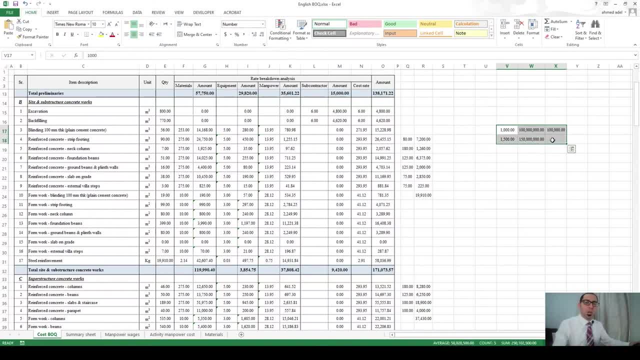 150 million. This is called the end unit method And this is a conceptual method. This is not a definitive or a deterministic method. It is not accurate, guys, It is just an understanding. Okay, it will come somewhere around this, Maybe 50% more, maybe 50% less. Another example of this: a hospital. I did a. 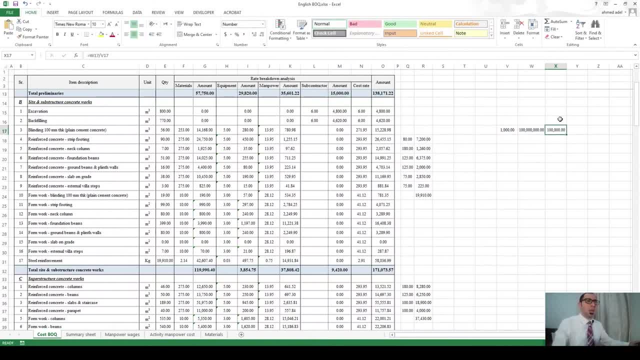 cost per one room. This divided by this, The room will be about 100,000.. So what if I have a new hotel that has 1500 rooms? 1500 rooms into the room price. So the new project will be about. 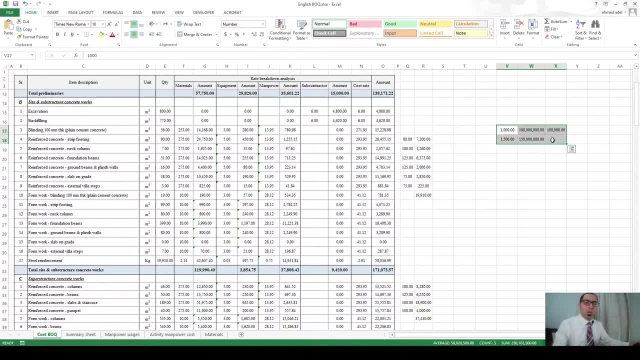 150 million. This is the cost of the room, So the cost of the room will be about 150 million. This is called the end unit method And this is a conceptual method. this is not a definitive or a deterministic method. It is not accurate, guys. It is just an understanding. Okay, it will come. 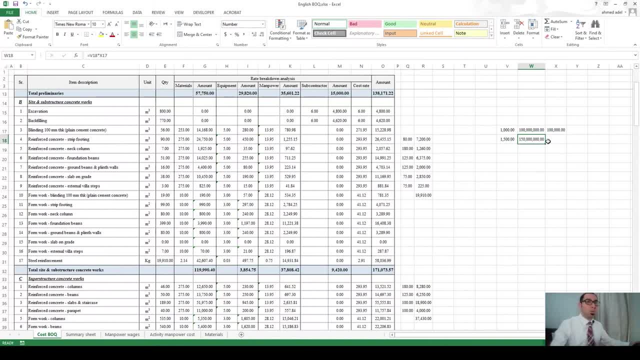 somewhere around this, maybe 50% more, maybe 50% less. Another example of this: a hospital I did, a hospital that has, let's say, 5000 beds at the cost of 500 million Again. So 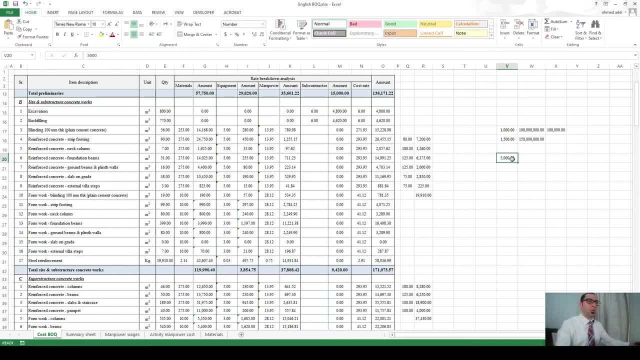 hospital that has, let's say, 5000 beds at the cost of, let's say, 500 million. Again, Let's say, 500 beds. I do not know how much each bed costed me. Again, 100,000.. So if I will make, 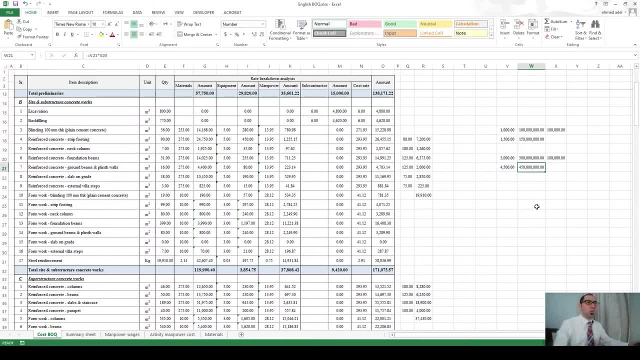 a new hospital that will have only 4500 beds, Then this one into this one, So it will be around 450 million. So this is the end units, How many units and how much the project, from the historical data, cost me And based on this knowledge, I will do in 30 seconds an estimate. Of course it's a 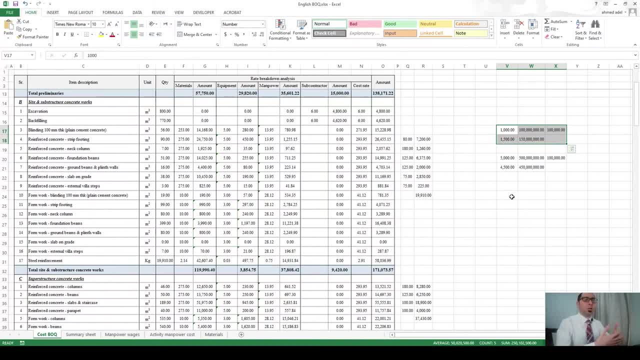 another way of the conceptual estimate, a method called the physical units. and physical units means what? let's say that I have a villa of 1,000 square meters, and the villa of 1,000 square meters costed me in the past 3 million. so per 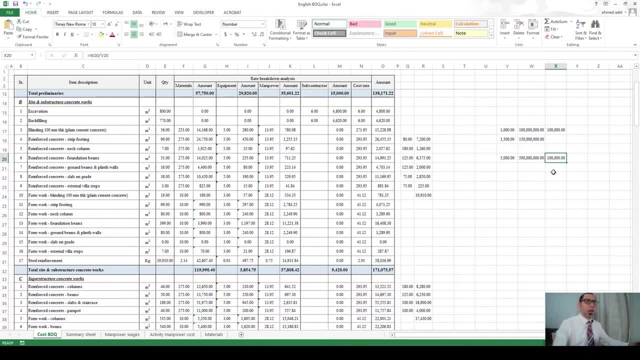 much. each bed costed me again hundred thousand. so if i will make a new hospital that will have only four thousand five hundred beds, then this one into this one. so it will be around 450 million. so this is the end units, how many units and how much the project from the historical data cost me. 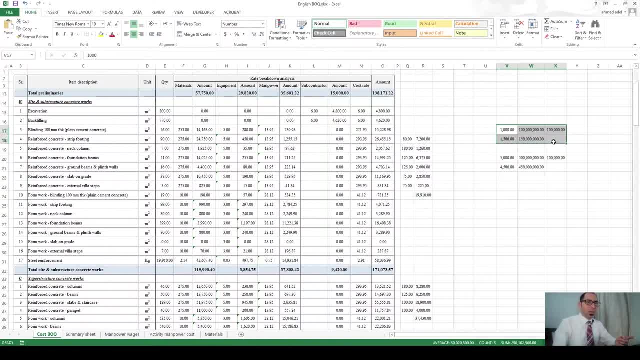 and, based on this knowledge, i will do in 30 seconds an estimate. of course it's a conceptual estimate. there is another way of the conceptual estimate, a method called the physical units. and physical units means what? let's say that i have a villa of one thousand uh square meters and the 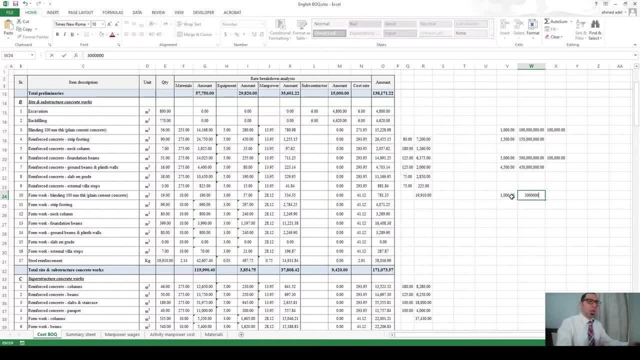 villa of one thousand square meters costed me in the past three million. so per each square meter, three million divided by thousand, so one square meter is three thousand dirhams or dollars or whatever the currency you are using. so if i have 850 villa, the 850 will be multiplied by the. 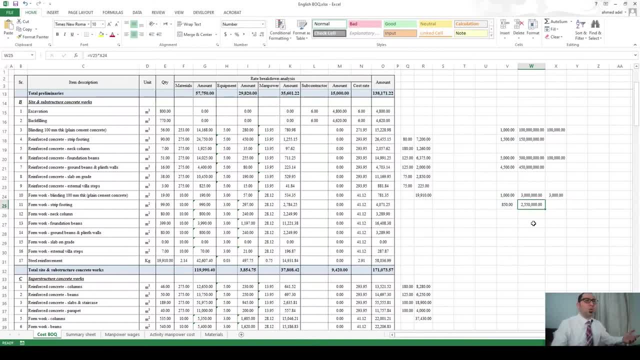 3000, which is the rate per square meter. so the new villa is 2.55 million. again, this is something conceptual we have not. we didn't go into the details to see what are the specifications of this villa, and what is the specifications of this villa if the requirements or specifications of the 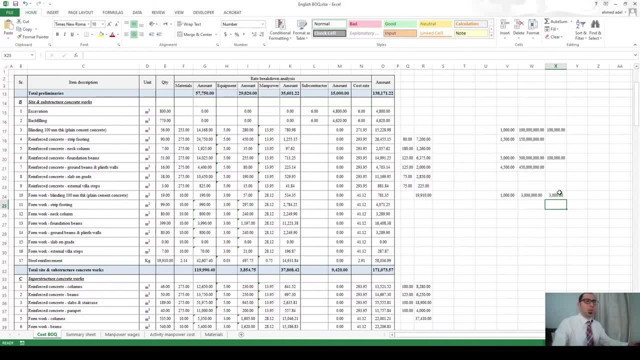 each square meter 3 million divided by thousand. so one square meter is 3,000 dirhams or dollars or whatever the currency you are using. so if I have 850 villa, the 850 will be multiplied by the 3,000, which is the rate per square meter. 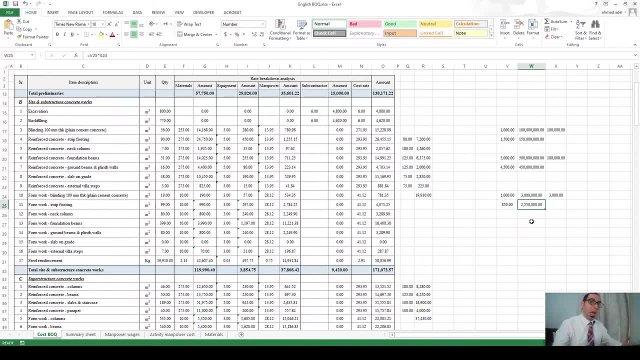 so the new villa is 2.55 million. again, this is something conceptual we have not. we didn't go into the details to see what are the specifications of this villa and what is the specifications of this villa if the requirements or specifications of the two projects are little bit near. 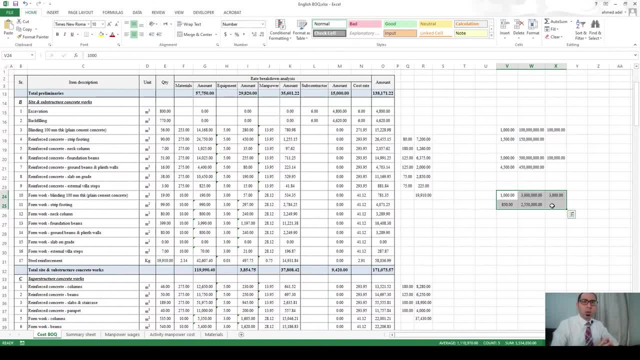 then these prices might be somewhere proper or near from the actual cost price. so all these methods are conceptual methods, and I just wanted to tell you what a conceptual method is. now let's delete this and let's go to the other part, which is the deterministic or definitive estimate. the definitive 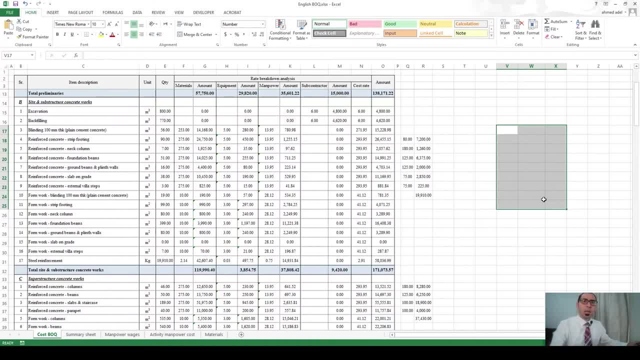 estimate is a very accurate estimate and actually it has five classes plus one, two, three, four and five. class five is the lowest in the accuracy and the class one is the highest in the accuracy. and what is the difference between each of these classes, starting from class one to class five? actually, the difference is: 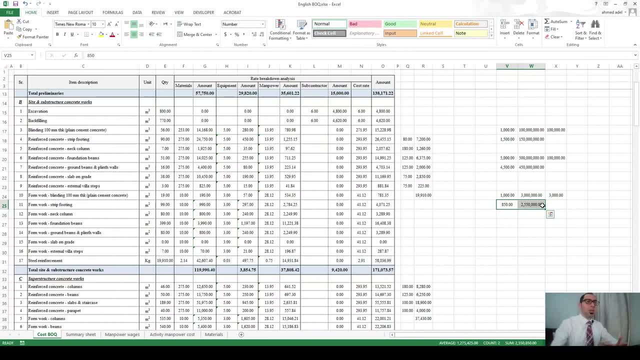 two projects are a little bit near, then these prices might be somewhere proper or near from the actual cost price. so all these methods are conceptual methods, and i just wanted to tell you what a conceptual method is. now let's delete this and let's go to the other part, which is the deterministic or definitive estimate, the 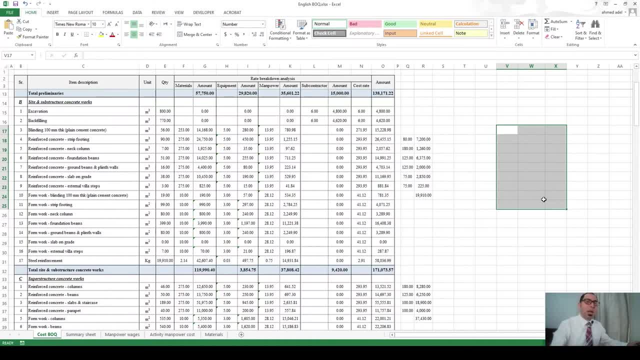 definitive estimate is a very accurate estimate and actually it has five classes plus one, two, three, four and five. class five is the lowest in the accuracy and the class one is the highest in the accuracy. and what is the difference between each of these classes, starting from class one to class five? 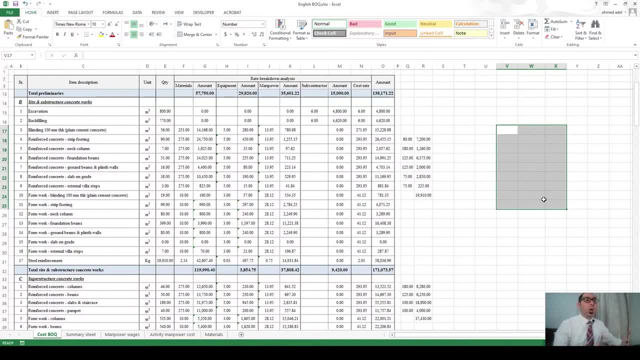 actually the difference is the project definition. what are the available data or information about the project? do we have all the drawings of the project? did we get quotations for all the work packages in the project from the specialists or from the subcontractors who will do these things? so, depending on the available information regarding the project, 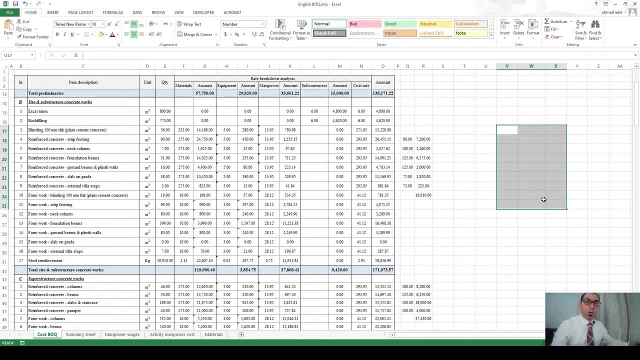 the accuracy or the class that we will use for a definitive estimate will be determined. so the most accurate class is class one where the available information is everything. i have everything available. i have drawings, i have specifications, i have soil report, i got quotations from subcontractors. i did everything. i have all the required information in order to 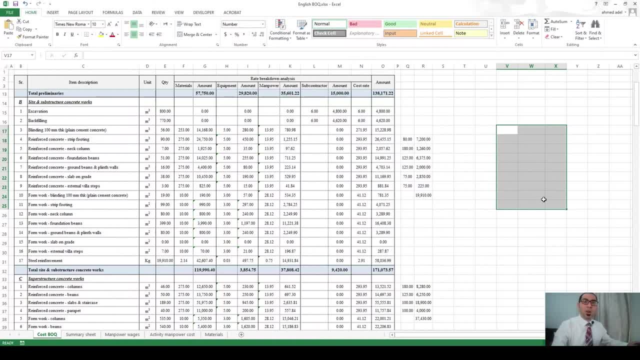 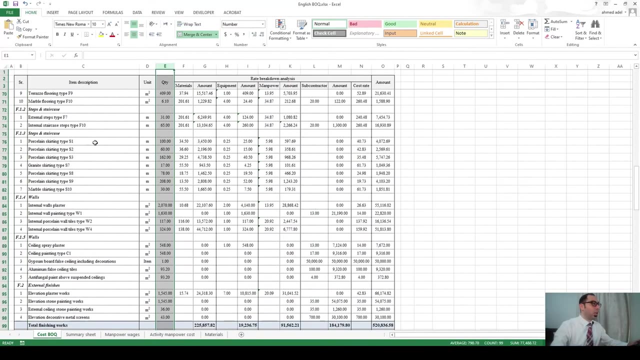 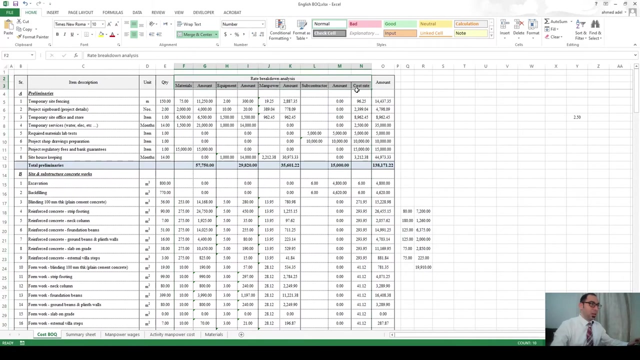 derive a correct or a class one definitive estimate. so let me give you an example here. this is a definitive estimate because we have full scope, we have like quantified everything and we have the quantities of each and every item. so now, if I just put a very accurate rate here, okay, I will get a. 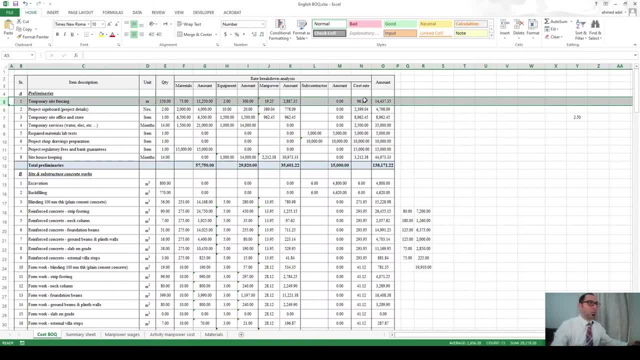 very accurate cost amount for this item, for example. so in order for me to put a very accurate rate here, what I will do, I want to know the breakdown. what are the things or the cost elements included in this rate? what are the cost elements included in this rate? and the cost elements will be material equipment. 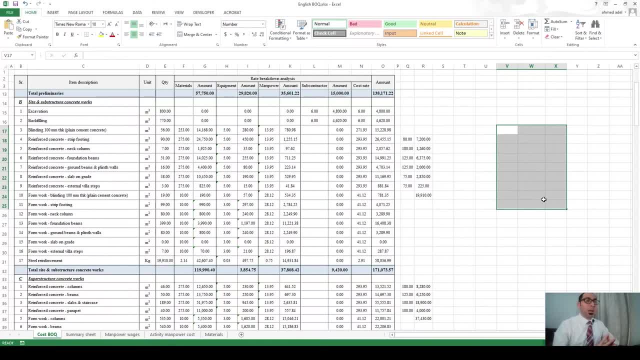 the project definition? what are the available data or information about the project? do we have all the drawings of the project? did we get quotations for all the work packages in the project from the specialists or from the subcontractors who will do these things? so, depending on the available information regarding the project, the accuracy or the class that we 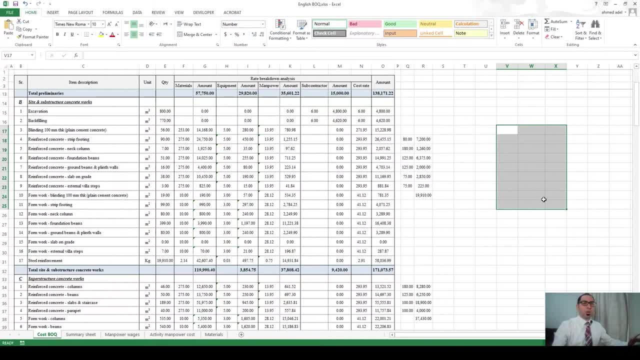 will use for a definitive estimate will be determined. so the most accurate class is plus one where the available information is everything. I have everything available. I have drawings, I have a specifications, I have soil report, I got quotations from subcontractors. I did everything. I have all the 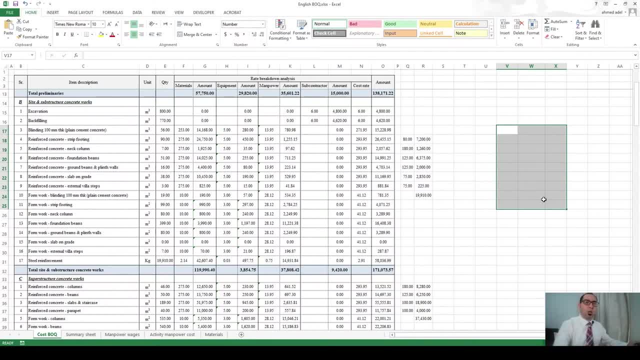 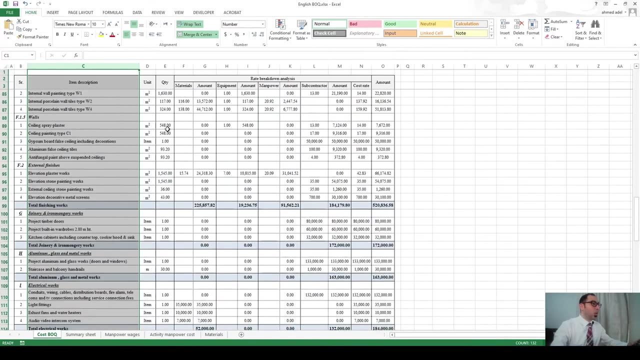 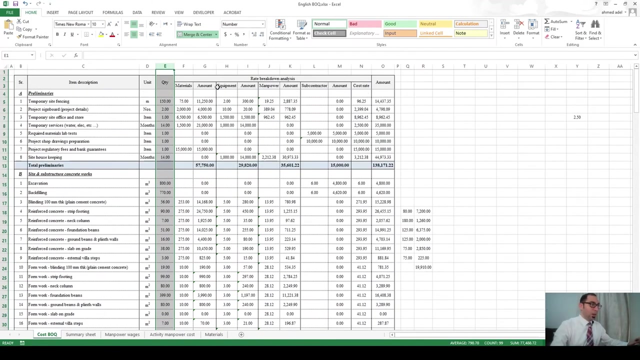 required information in order to derive a correct or a class one definitive estimate. so let me give you an example here. this is a definitive estimate because we have full scope, we have like quantified everything and we have the quantities of each and every item. so now, if I just put a very accurate rate here, okay, I will get a very accurate. 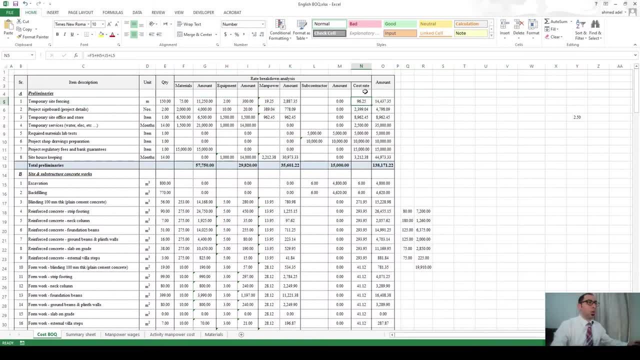 cost and for this item, for example. so in order for me to put a very accurate rate here what I will do, I want to know the breakdown. what are the things or the cost elements included in this rate? what are the cost elements included in this rate? and the cost elements will be material equipment, manpower and 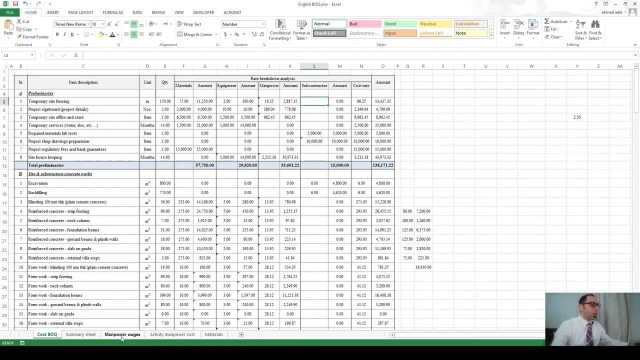 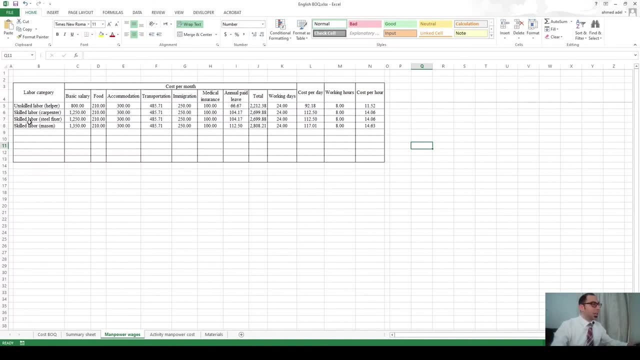 subcontractor. so I will be starting with, let's say here: these are the calculations of manpower: skilled and unskilled laborers. I want to calculate how much is the cost per day and how many working hours per day and what is the cost per hour. this is the first element, guys, I want to understand each. 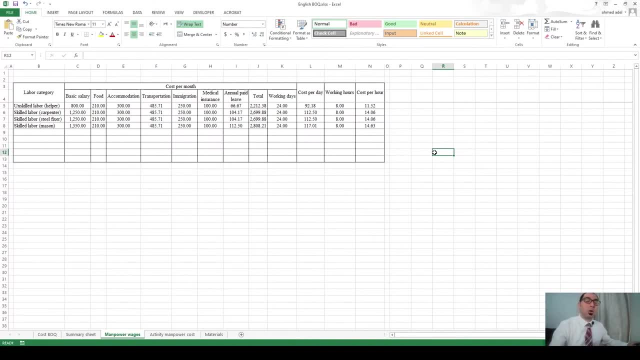 labor in my company. how much is he costing me per day and how much is he costing me per hour and why I need this information? because if I know how much he is costing me per day and what can he do per day, so i can get the rate per unit of measurement. for example, if this skilled 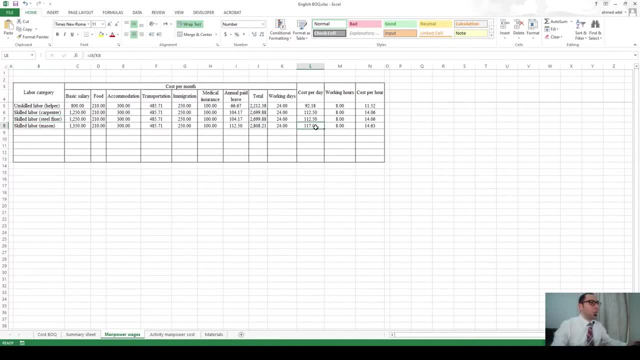 labor here, mason, if he's costing me per day 117 and he can produce 25 square meters, for example, of any item, so each square meter in terms of manpower, how much is it costing me? i will say 117 divided by 25, i will pay to this labor 117 and he will give me 25 meters. so that means that 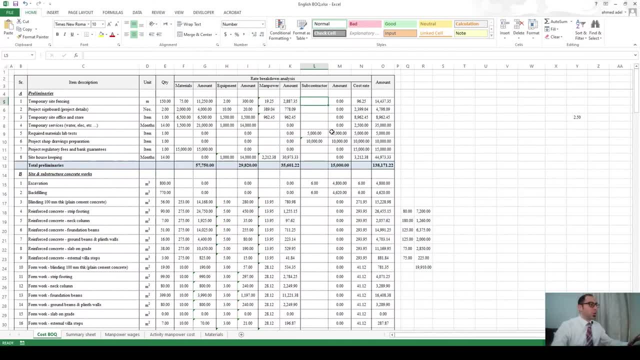 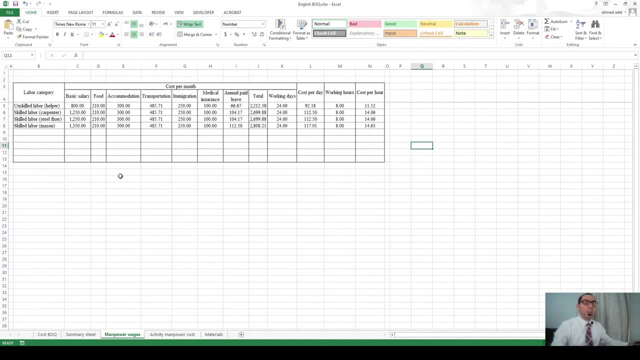 manpower and subcontractor. so I will be starting with, let's say here: these are the calculators of manpower, skilled and unskilled laborers. I want to calculate how much is the cost per day and how many working hours per day and what is the cost per. 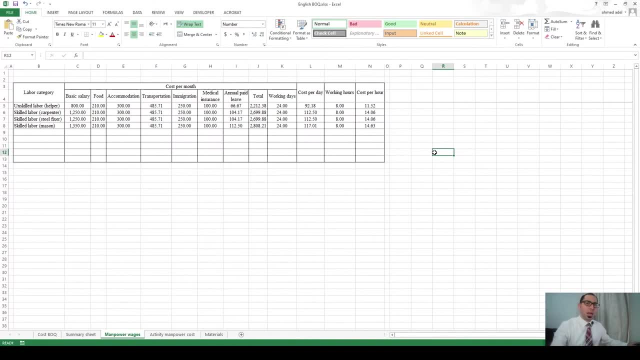 hour. this is the first element, guys. I want to understand each labor in my company. how much is he costing me per day and how much is he costing me per hour, and why? I need this information? because if I know how much he is costing me per day, 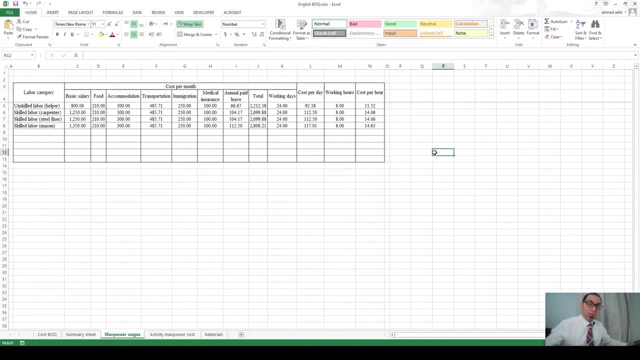 and what can he do per day so I can get the rate per unit of measurement. for example, if this skilled labor here, Mason, if he's costing me per day 117 and he can produce 25 square meters, for example, of any item, so each square meter in 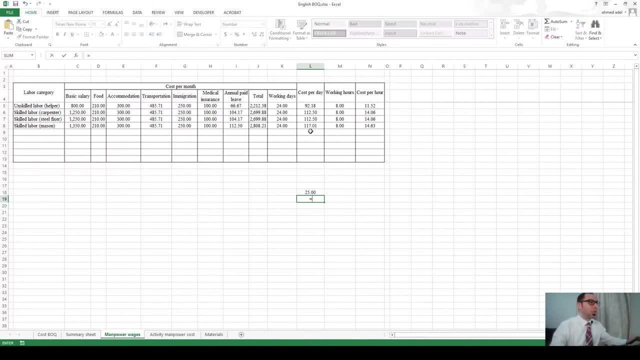 terms of manpower. how much is it costing me? I will say 117 divided by 25. i will pay to this labor 117 and he will give me 25 meters. so that means that this 117 did a job for me of 25 meters. so how much each meter of these 25 meters costed me? it costed me. 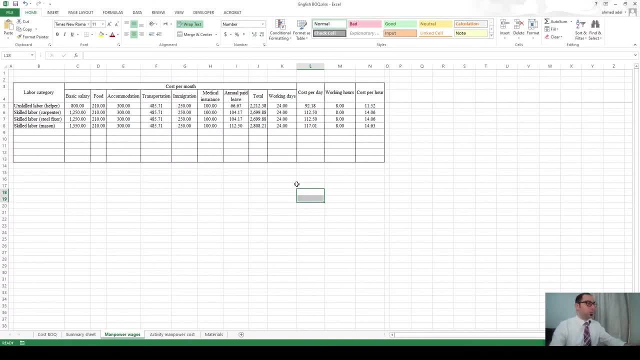 4.68. and from this calculation sheet, for example, we have the categories of labor. here we have how much his basic salary. food, accommodation, if i am providing accommodation, if i am providing transportation- in some countries there are some immigration or visa fees paid yearly or every two years. if there is a medical insurance, if, as per his labor contract, i have to. 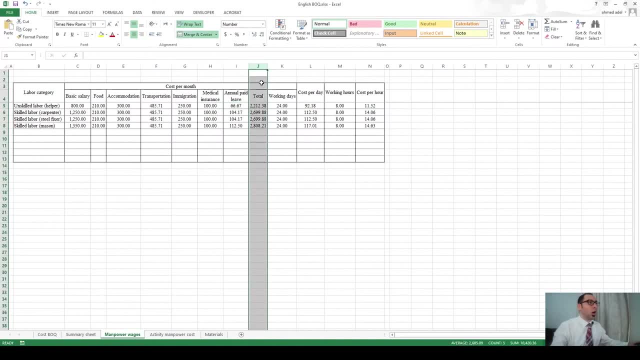 give him one month paid leave, for example. so how much is he costing me in terms of everything- salary plus food, plus accommodation, plus everything- how much this labor is costing me per month and how many working days is he working per month? so when you divide the total cost of labor, divided by the number of working days, you get how much is he costing you. 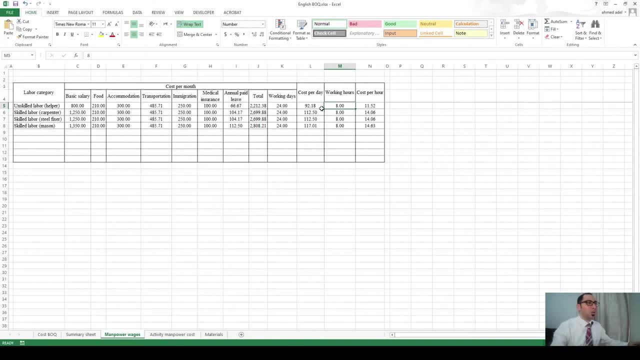 per day and if he is working eight hours per day. so when you divide the 92 divided by the number of hours, or the cost per day divided by the number of hours, you get the cost per hour. and i actually need these two columns to go to the next step, which is productivity. so here i have something called activity manpower. 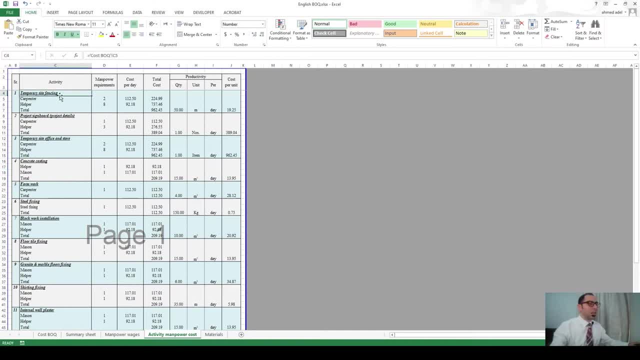 cost. let's say that i want to do a temporary site fencing around my plot or site or project. i want to do a temporary fencing. so for this temporary fencing i need two carpenters and i need eight helpers. and i know that these two, that these 10 people, i know that these 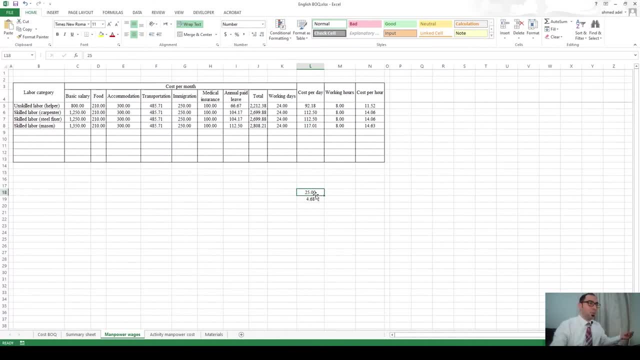 this 117 did a job for me of 25 meters. so how much each meter of these 25 meters costed me? it costed me 4.68 and from this calculation sheet, for example, we have the categories of labor. here we have how much his basic salary, food, accommodation, if i am providing accommodation, if 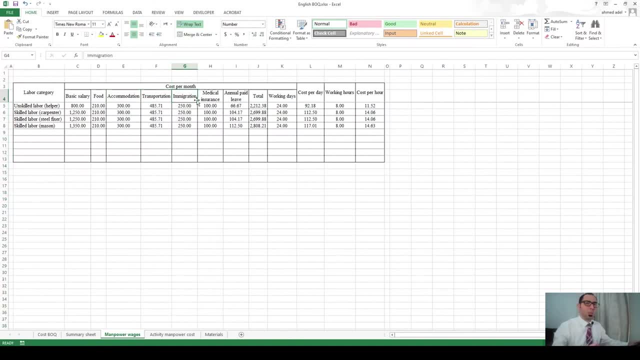 i am providing transportation in some countries. there are some immigration or visa fees paid yearly or every two years if there is a medical insurance, if, as per his labor contract, i have to give him one month paid leave, for example. so how much is he costing me in terms of everything? 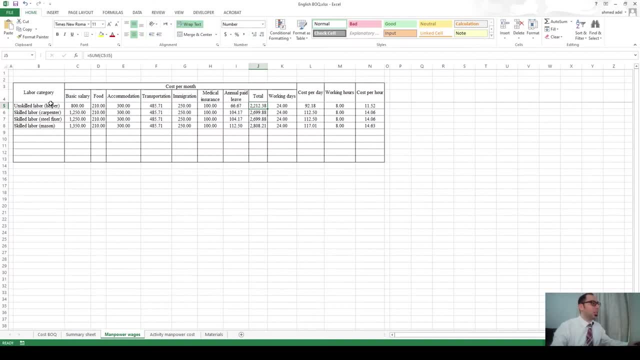 salary plus food, plus accommodation, plus everything, how much this labor is costing me per month and how many working days is he working per month. so when you divide the total uh cost of labor, divided by the number of working days, you get how much is he costing you per day, and if he is working eight hours per day. so when you divide, 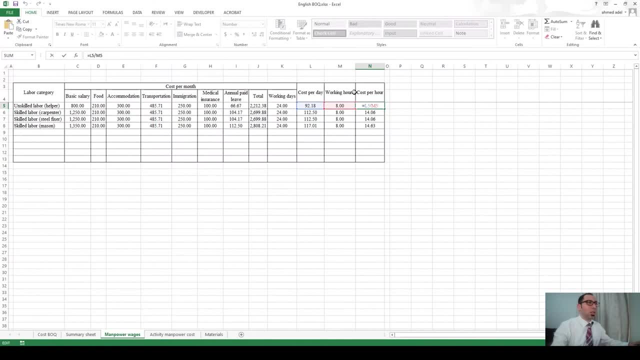 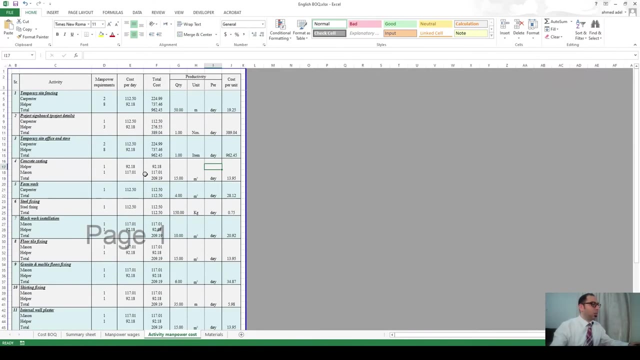 the 92 divided by the number of hours, or the cost per day divided by the number of hours, you get the cost per hour. and i actually need these two columns to go to the next step, which is productivity. so here i have something called activity manpower cost. let's say that i want to do a temporary site fencing around my plot or site or project i want. 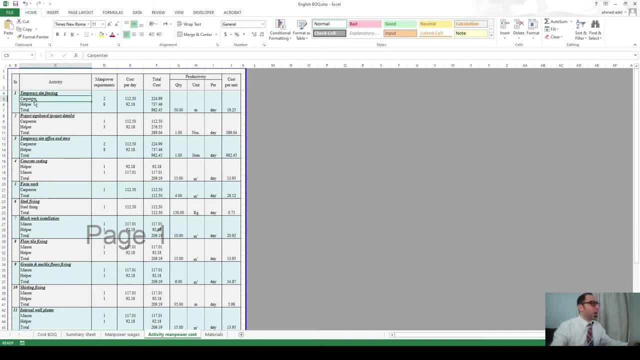 to do a temporary fencing. so for this temporary fencing i need two carpenters and i need eight helpers, and i know that these two, that these 10 people, i know that these 10 people can install like 50 linear meters of temporary fencing per day. so first, 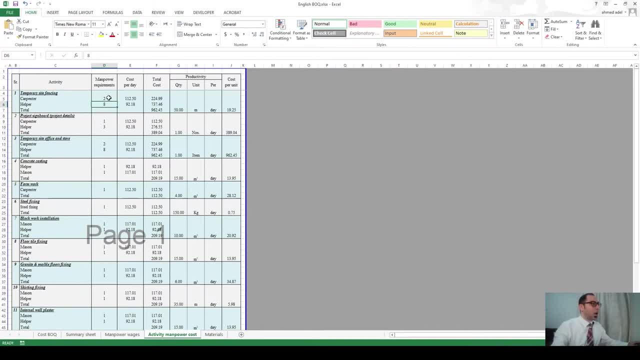 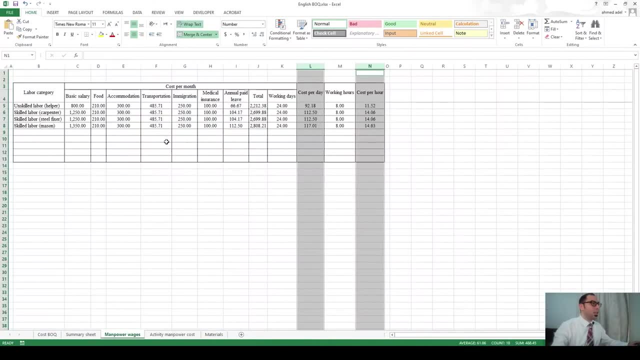 of all these 10 labors, two carpenter and eight helpers, how much they will cost me per day? two of them, the carpenter, will cost me per day as per these calculations here. this is the carpenter, for example. we calculated his salary and his everything and the cost per day is 112.. so this cost per day. 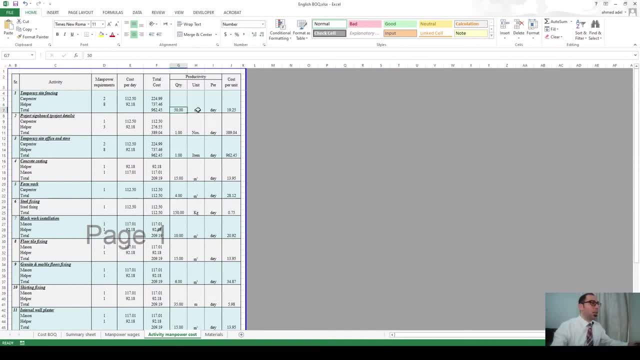 10 people can install like 50 linear meters of temporary fencing per day. So, first of all, these 10 laborers, 2 carpenters and 8 helpers, how much they will cost me per day? Two of them, the carpenter, will cost me per day as per these calculations here. 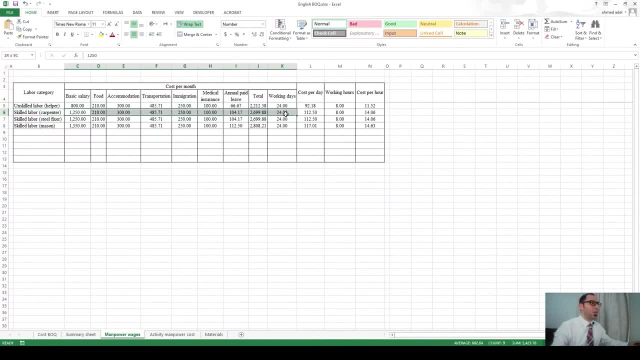 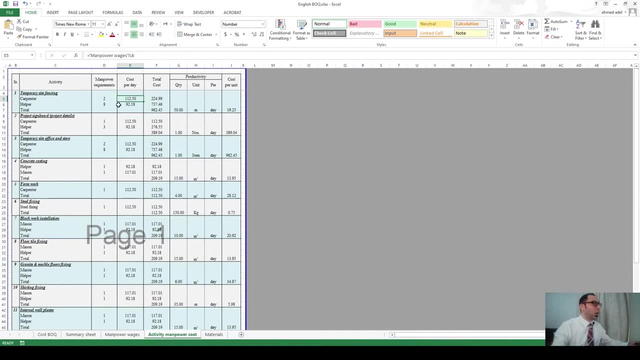 This is the carpenter, for example. we calculated his salary and his everything and the cost per day is 112. So this cost per day will come here 112 and the helper, similarly, is costing me 92. So I need 2 carpenters into 112, it will be 224, and 8 laborers into 92 per day it will. 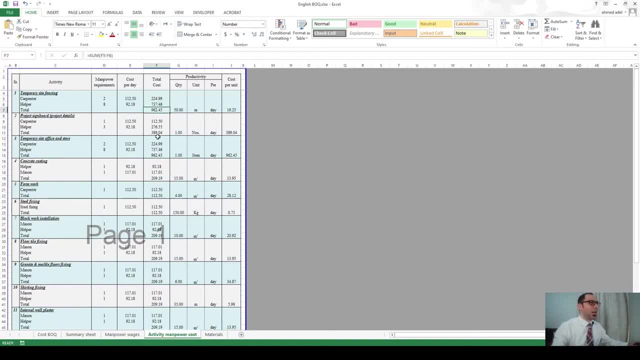 be 737.. So this plus this is 962.. These 10 laborers will cost me as a company per day, 962 or 963.. Okay, this is how much they will cost me, But what can they give me in return? Like which work they can do in one day. 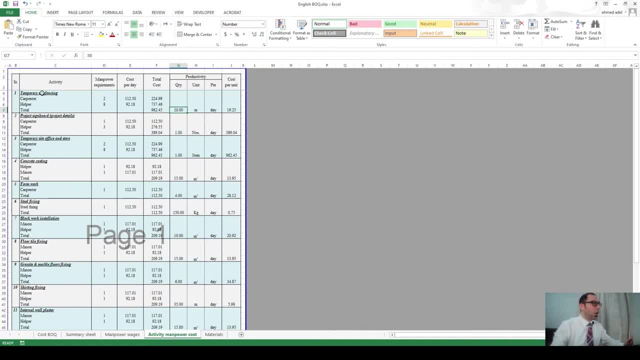 This is called here the productivity. They can install a temporary fencing: 50 linear meters per day. That means that each cost per unit is how much they will cost me and which quantity they can do per day. So this divided by this, So I will see that each linear meter in terms of manpower is costing me 92.. 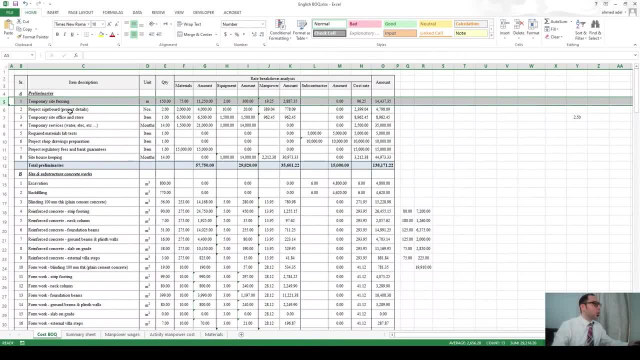 19.25. okay, So here, when I come to my BOQ, I have this item which is temporary site fencing, and how many linear meters I have. I have 150 linear meters of temporary site fencing. okay, So in terms of manpower, okay for these 150 meters, for, in terms of manpower, each meter. 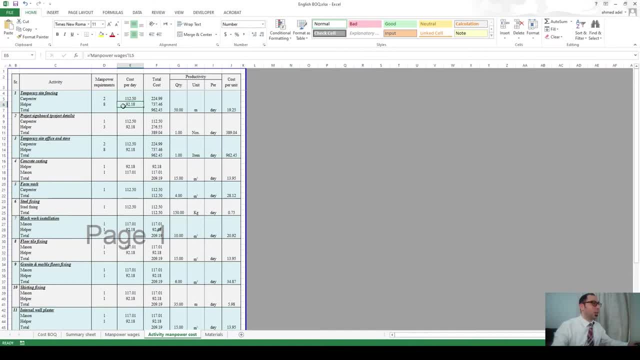 is 112.. so the cost per day is the same as the cost per day i have my company and the other carpenters will come here- 112, and the helper, similarly, is costing me 92.. so i need two carpenters into 112, it will be 224, and eight labors into 92 per day, it will be 737. so this 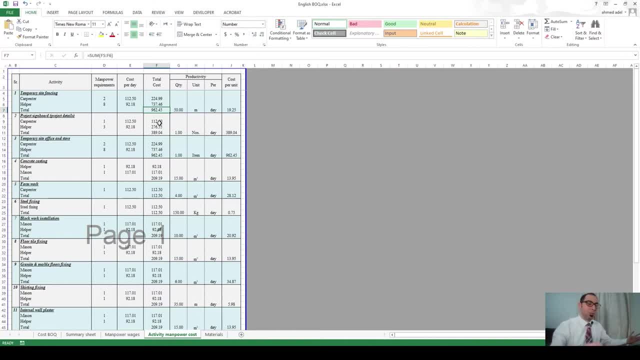 plus this is 962. these 10 laborers will cost me, as a company per day, 962 or 963. okay, this is how much they will cost me, but what can they give me? okay, this is how much they will cost me, but what can they give me. 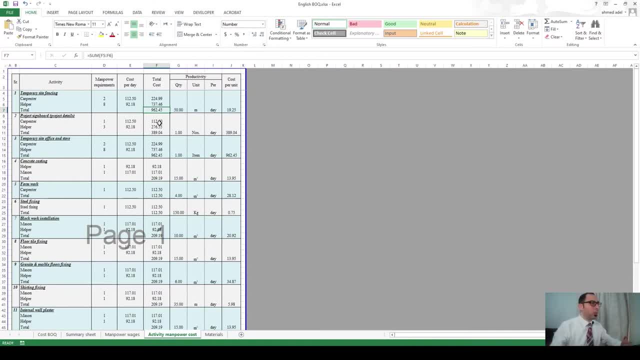 me in return, like which work they can do in one day. they can this. this is called here the productivity. they can install a temporary fencing- 50 linear meters per day. that means that each cost per unit is how much they will cost me and which quantity they can do per day. so this divided by 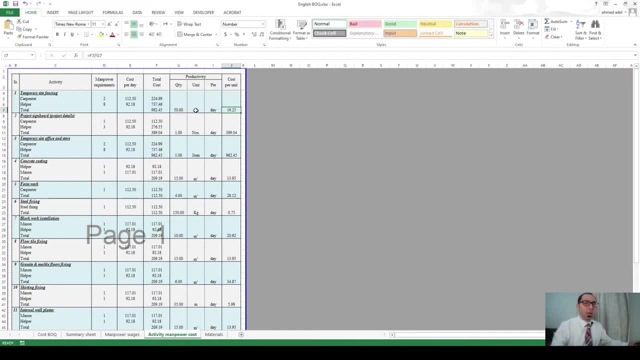 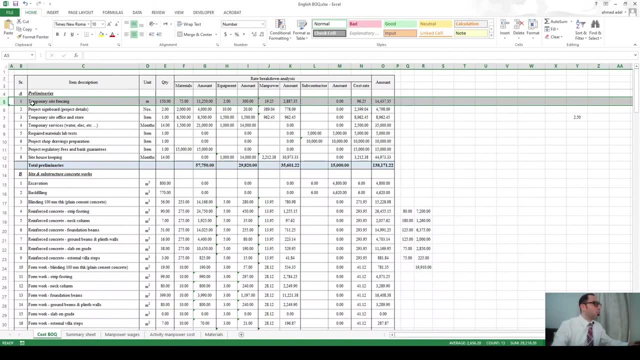 this. so I will see that each linear meter in terms of manpower is costing me 19.25. okay, so here, when I come to my BOQ, I have this item which is temporary site fencing and how many linear meters I have. I have 150 linear meters of temporary site fencing. okay so, in terms of manpower, okay for these. 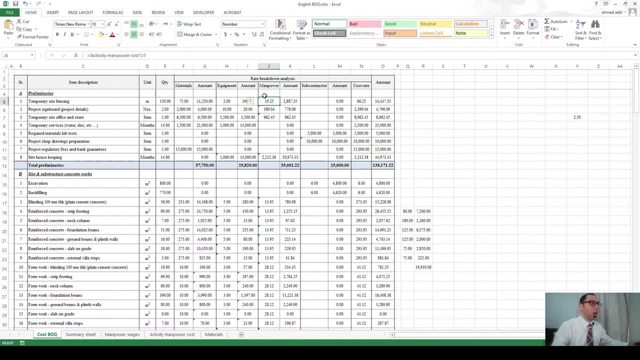 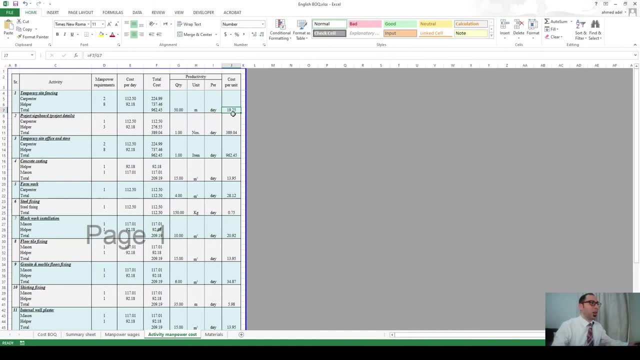 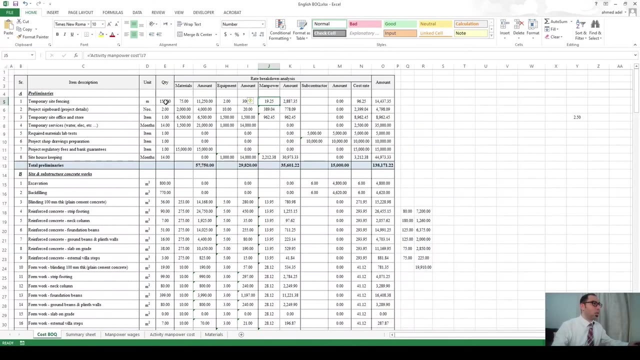 150 meters for, in terms of manpower each meter, how much it will cost me for the installation. I just calculated this here, which is 19.25 cost per unit, like 19.25 per linear meter. so if I want to install 150 linear meters multiplied by, 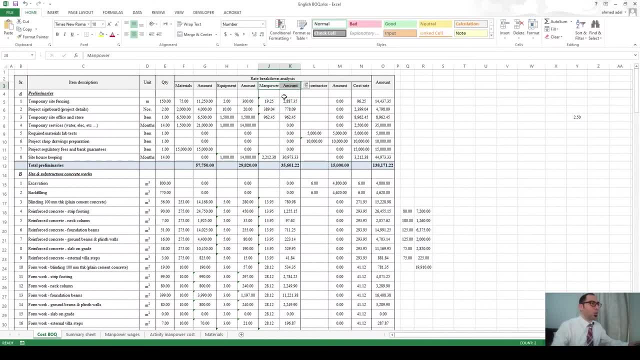 19.25. this is the amount. so in terms of manpower to install the site fencing, I need 2887. okay, what about the materials itself? guys, if I want to install a temporary site fencing, I have to buy it. I have because the quantity is 150 linear. 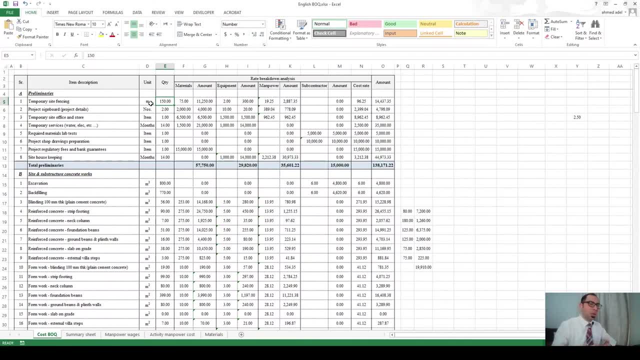 meters. so I need to buy 150 linear meters of temporary site fencing. okay, but when I go to the seller or to the vendor or to the supplier and I say I want a temporary site fencing, how much per linear meter, he will give me a quotation or he will give me a proposal of 75 dirhams or dollars. 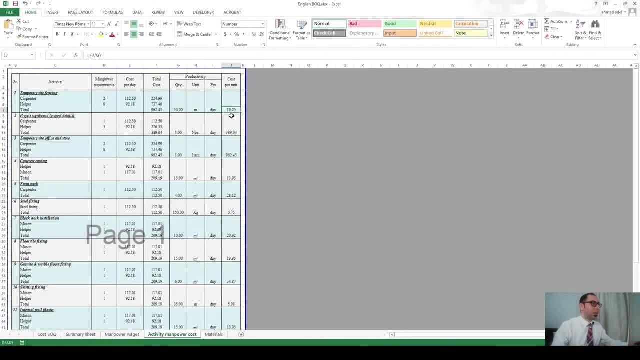 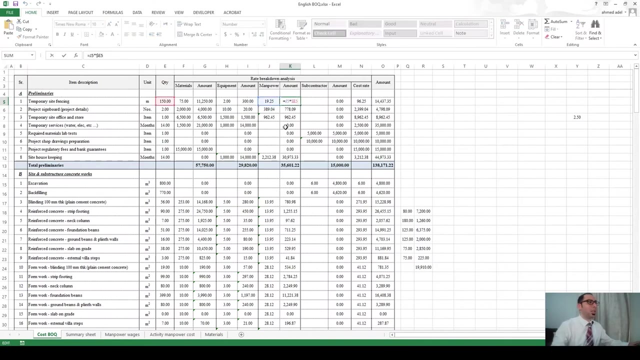 how much it will cost me for the installation. I just calculated this here, Which is 90.. 19.25 cost per unit, like 19.25 per linear meter. So if I want to install 150 linear meters multiplied by 19.25, this is the amount. 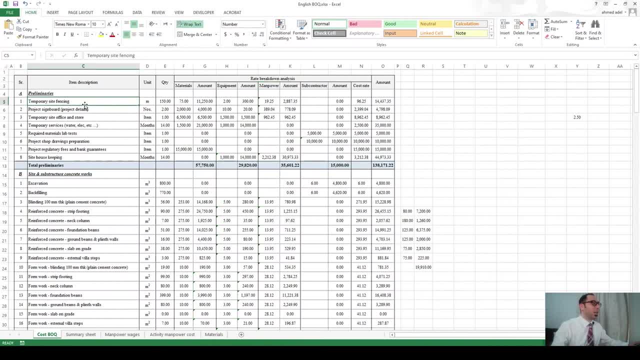 So, in terms of manpower to install the site fencing, I need 2887. okay. What about the materials itself? Guys, if I want to install a temporary site fencing, I have to buy it. I have because the quantity is 150 linear meters. So I need to buy 150 linear meters of temporary site fencing, okay? 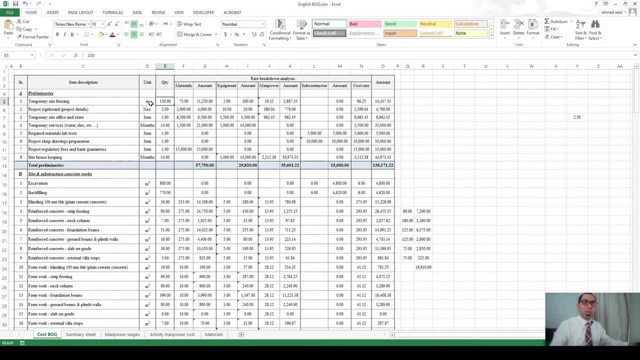 But when I go to the seller or to the vendor or to the supplier and I say I want a temporary site fencing, how much per linear meter, he will give me a quotation or he will give me a proposal of 75 dirhams or dollars or whatever currency per linear meter. 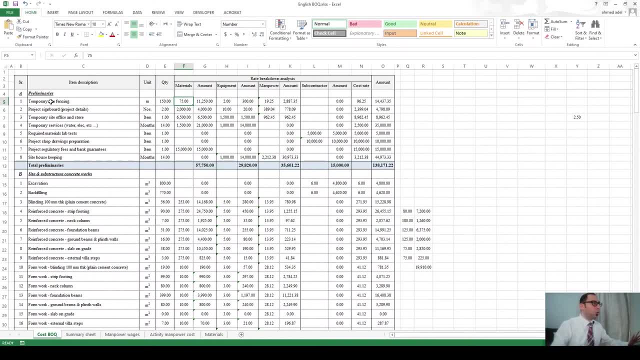 So this is the cost of the material. So in order to do a temporary site Fencing 150 linear meters, I need to buy each linear meter. I'll buy the materials by 75, let's say whatever currency, and I will install each linear meter. 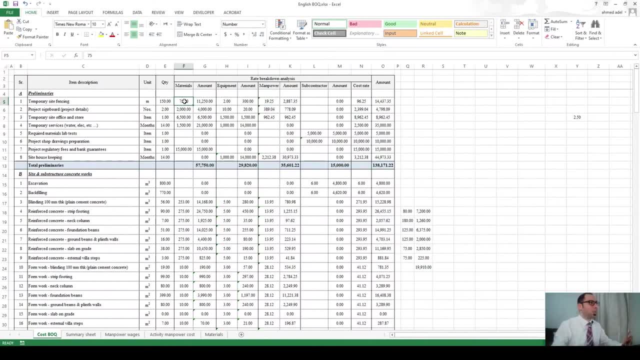 by 19.25. okay, So this is regarding the materials. and again here for the materials, when I multiply the supply rate, when multiplied by the quantity, it gives the amount. then for the manpower, when I multiply the 19.25 by the quantity, Again it gives the amount. so I'll buy this fence by the 150 meters will cost me as a material. 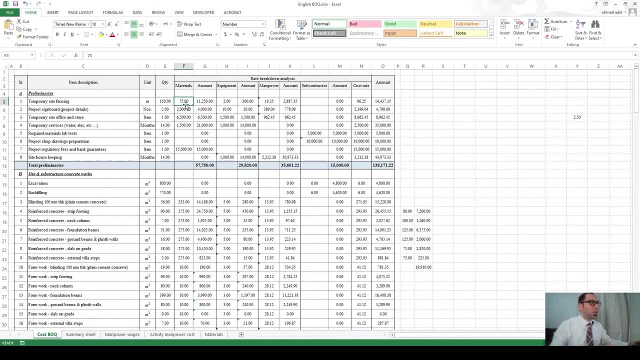 or whatever currency, per linear meter. so this is the cost of the material. so, in order to do a temporary site fencing 150 linear meters, i need to buy each linear meter. i'll buy the materials by 75- let's say whatever currency- and i will install each linear meter by 19.25. okay, so this is regarding the materials. 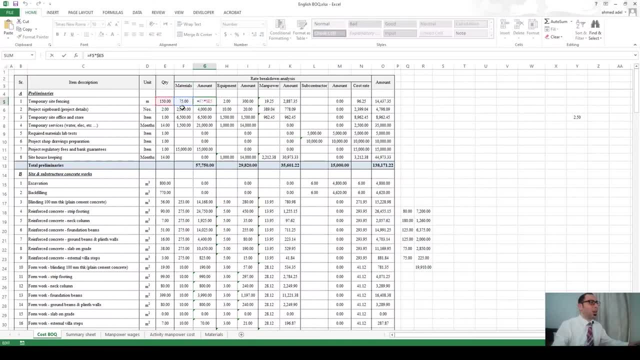 and again here for the materials, when i multiply the supply rate, when multiplied by the quantity, it gives the amount. then for the manpower, when i multiply the 19.25 by the quantity, again it gives the amount. so i'll buy this fence by the 150 meters will cost me as a material. 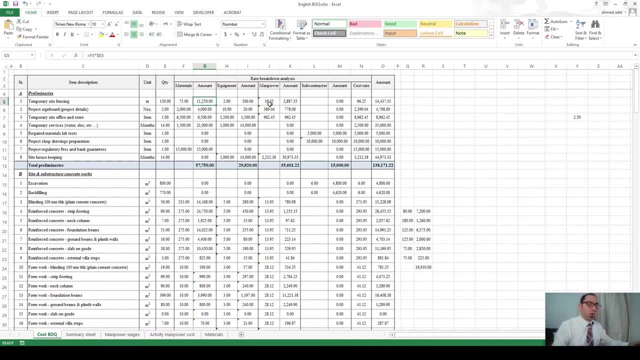 11 250 and the installation or the manpower will be 2888. but these laborers who will do the installation of these materials, they need some equipments. they need maybe some hammers or some nails or something like that. guys, i know that everyone wants to be very accurate or as much accurate as 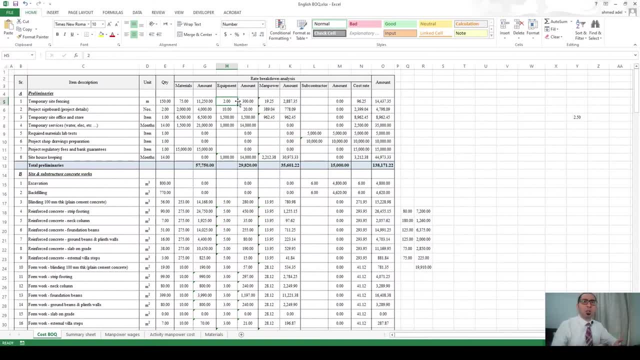 you can be, but still there is a limit that you cannot go beyond, like here. how, how i will know, in terms of equipment or tools, how much each linear meter of this temporary site fencing will cost me, i have no idea. of course, it is something very hard to to estimate. so, in that, 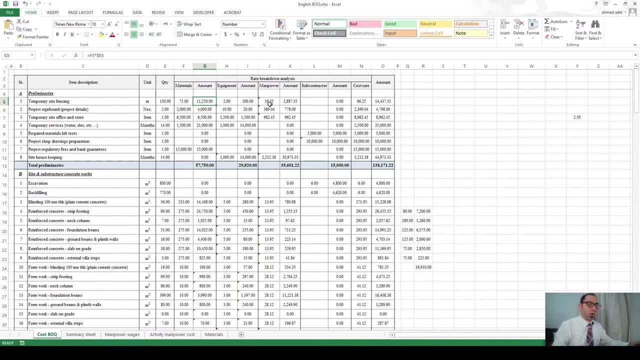 11,250 and the installation or the manpower will be 2,888.. But these laborers who will do the installation of these materials, they need some equipments. they need maybe some hammers or some nails or something like that. guys, I know that everyone. 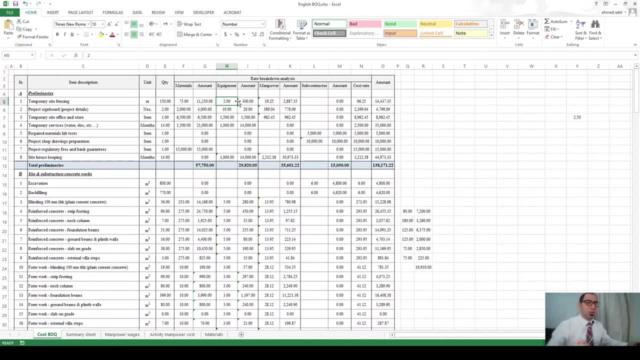 wants to be very accurate, Or as much accurate as you can be, but still there is a limit that you cannot go beyond, like here. how, how I will know, in terms of equipment or tools, how much each linear meter of this temporary site fencing will cost me. I have no idea. of course, it is something very 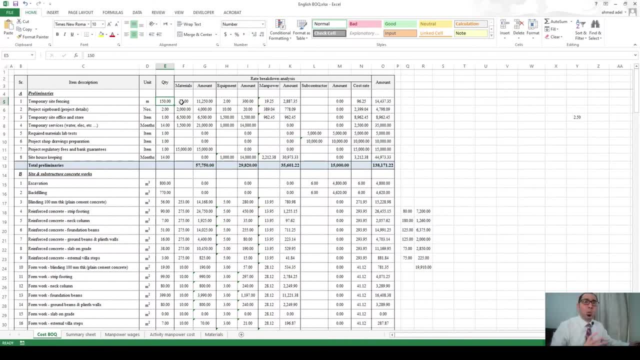 hard to estimate. So in that case we do something that called allowance- you allow. you allow for doing this part of the work or for this thing, Like here, when we talk about the tools or equipments required, I am allowing two dirhams or two dollars for each linear meter of the temporary site fencing. 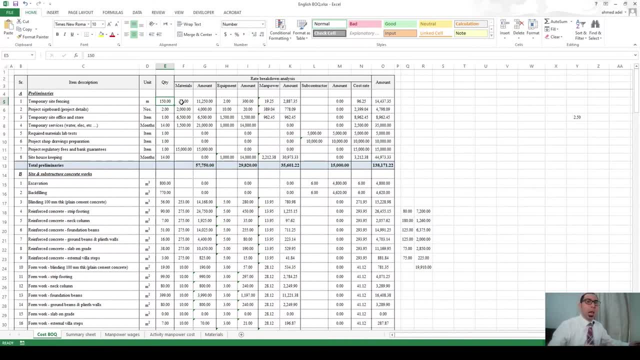 case we do something that called allowance. you allow, you allow for doing this part of the work or for this thing, like here. when we talk about the tools or equipments required, i am allowing two dirhams or two dollars for each linear meter of the temporary site fencing. so when i multiply the two, multiplied by the quantity, which is 150, 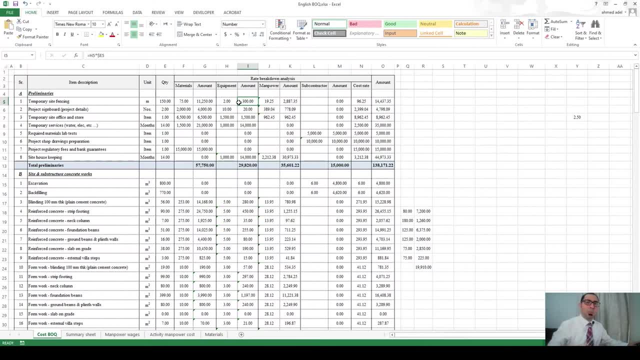 the amount is 300, so i am allowing an amount of 300 currency for the purchase or for the tools or for the equipments to be used to install this temporary site fencing. So we spoke about material, we spoke about equipment or tools, we spoke about manpower. Now subcontractor. Subcontractor is when you go and you outsource part of the works, Like if you are a contracting company. if you are a main contractor, you will do some of the activities you will do them in-house and some of the activities you will sublet or subcontract them to other companies to do it. 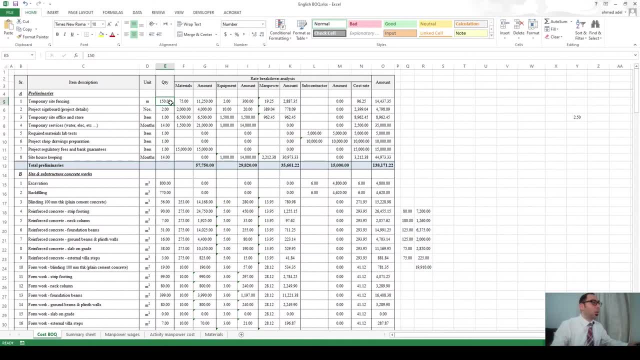 So when I multiply the two, multiplied by the quantity, which is 150, the amount is 300. so I am allowing an amount of 300 currency for the purchase or for the tools or for the equipments to be used to install This temporary site fencing. 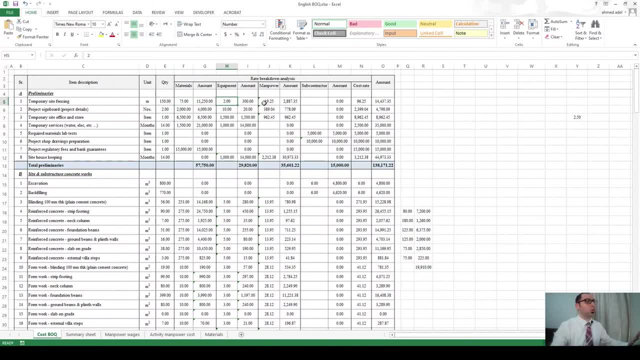 So we spoke about material, we spoke about equipment or tools, we spoke about manpower. Now, subcontractor. subcontractor is when you go and you outsource part of the works, like if you are a contracting company. if you are a main contractor, you will do some of the 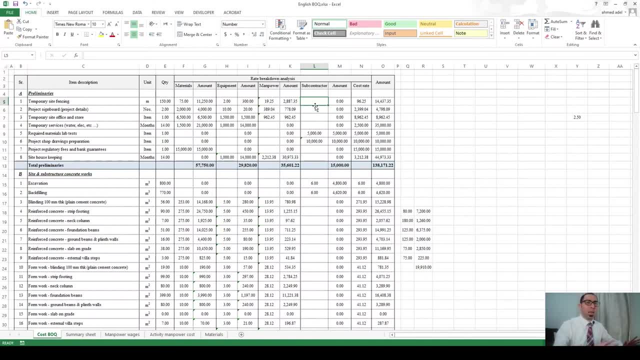 activities you will do them in house, and some of the activities you will sublet or subcontract them to other companies to do it. So, for example, here, when I am doing the estimation, there is something called the basis of estimate, and this is simply a list of assumptions that you have done in order to derive your estimate. 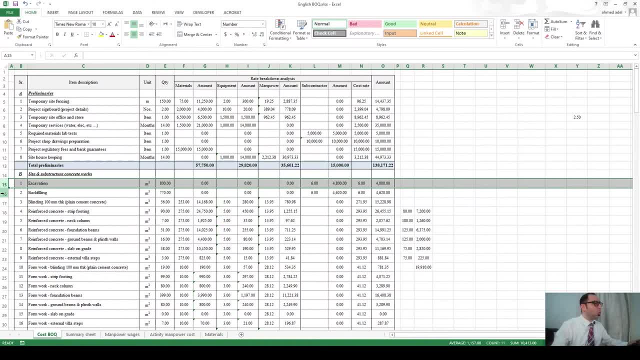 from. So my assumption here that I am going to do the excavation and back filling by a subcontractor, I'll just go a higher one guy. I'll just go and hire one guy who has some trucks, who has some excavators, and I'll give him their cubic meter of excavation. 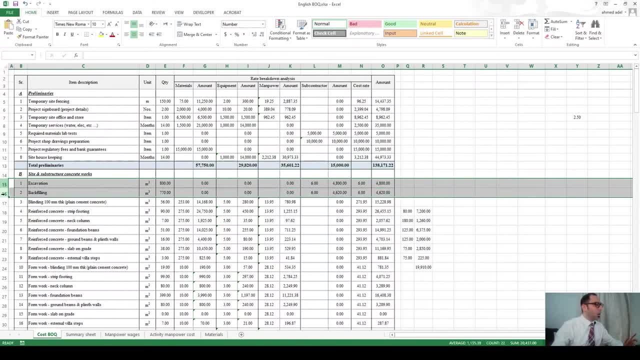 So, for example, here, when I am doing the estimation, there is something called the basis of estimate And this is simply a list of assumptions that you have done in order to derive your estimate from. So my assumption here that I am going to do the excavation and backfilling by a subcontractor. 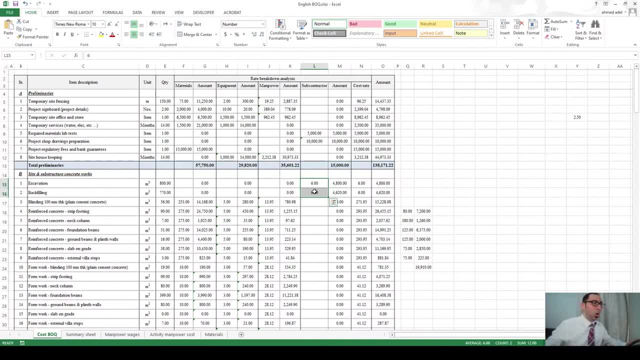 I'll just go a higher one. I'll just go and hire one guy who has some trucks, who has some excavators, and I'll give him per cubic meter of excavation and backfilling. And this price should be obtained from the market via vendor or subcontractor quotation. 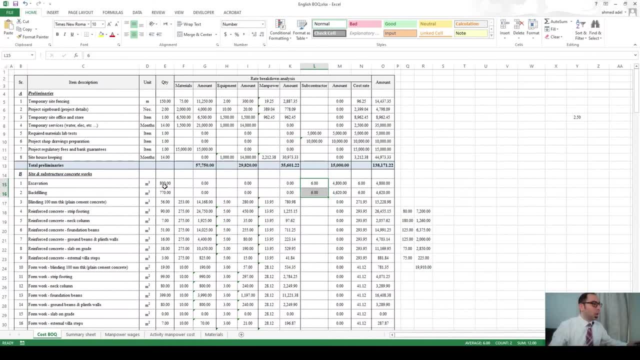 You will approach the subcontractor: Hi, I have a project and I have about 800 cubic meters of excavation and 770 cubic meters of backfilling. Please give me your price. He will tell you all right, per cubic meter. 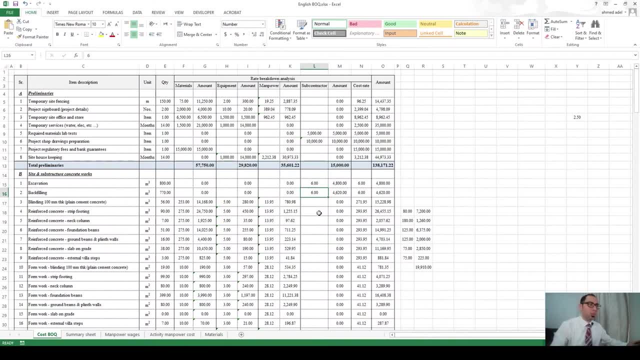 So here we have the number of excavations: 6- and backfilling 6 as well. So that means when I multiply the six by the quantity, it gives this amount for the excavation and this amount for the backfilling. And if the item requires you, as a company, to provide any tools or equipment, 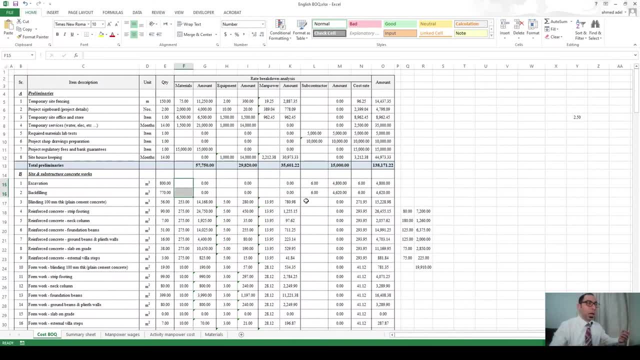 or any manpower or any materials to help this subcontractor to do his job. you have to put these things here, But in this case, or in the case of these trucks, In the case of these two items, I don't need anything. 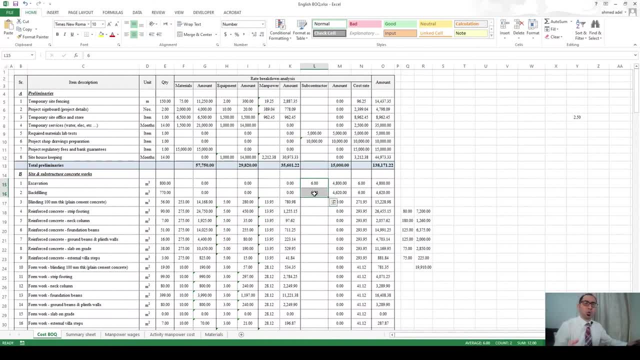 Excavation and back filling, and this price should be obtained from the market via vendor or subcontractor quotation. You will approach the subcontractor. hi, I have a project and I have about 800 cubic meters of excavation and 770 cubic meters of back filling. 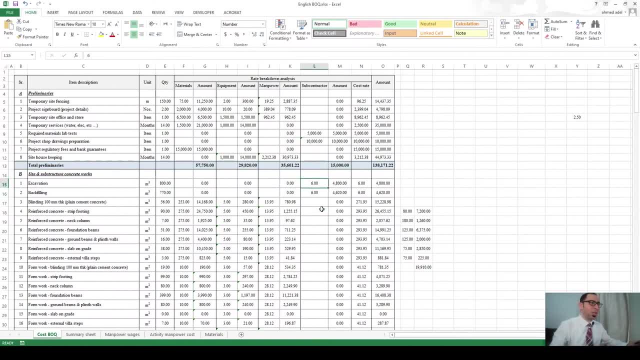 Please give me your price. He will tell you all right. per cubic meter of excavation, six and back filling six as well. So that means, when I multiply the six by the quantity, it gives this amount For the excavation and this amount for the back filling. and if the item requires you, 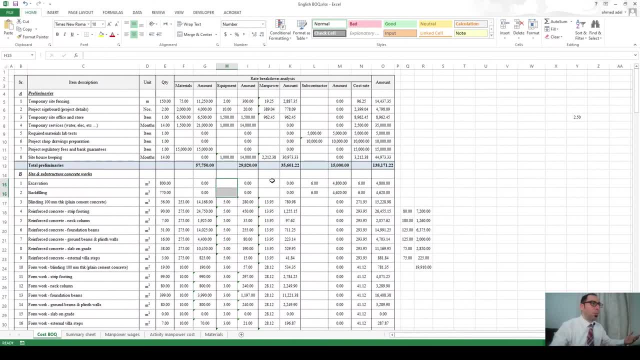 as a company, to provide any tools or equipments or any manpower or any materials to help this subcontractor to do his job. you have to put these things here, But in this case, or in the case of these two items, I don't need anything. He will just come, he will excavate, he will dispose, he will do everything. 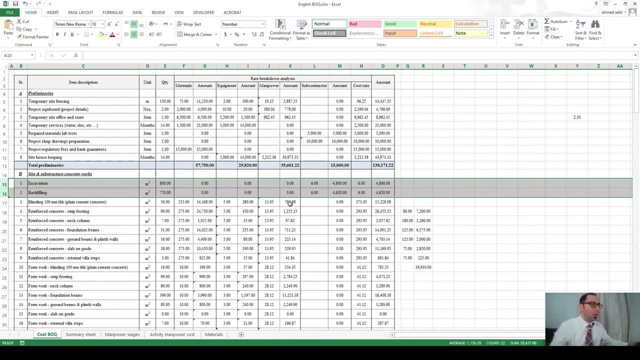 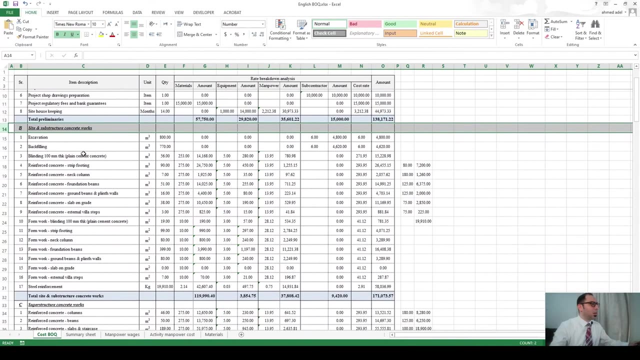 He will just come, he will excavate, he will dispose, he will do everything. I don't have to help him with any means. So if we now, if we go to the BOQ divisions which we have here, prelims, then site works and concrete works. 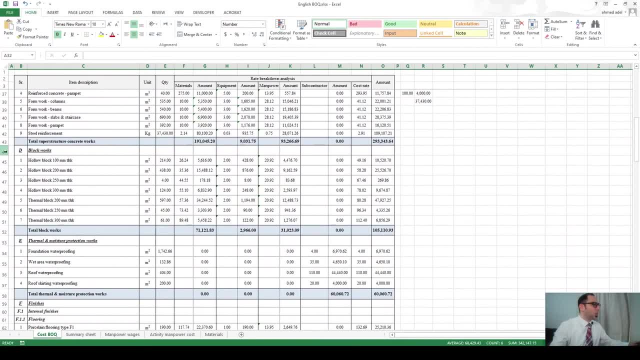 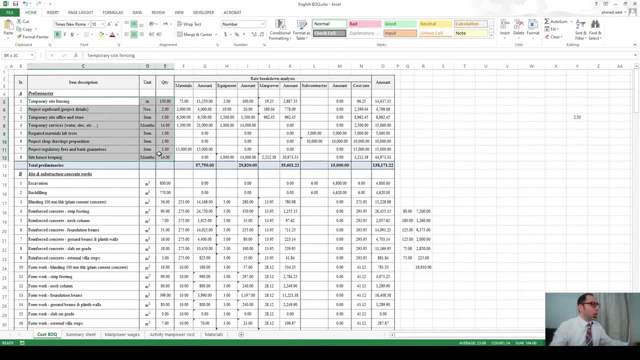 and then we have again superstructure works, block work, thermal and moisture finishes and all of that. Now, if you can see, guys, all these BOQ items, for each and every item I put here how much the material of this item will cost me. 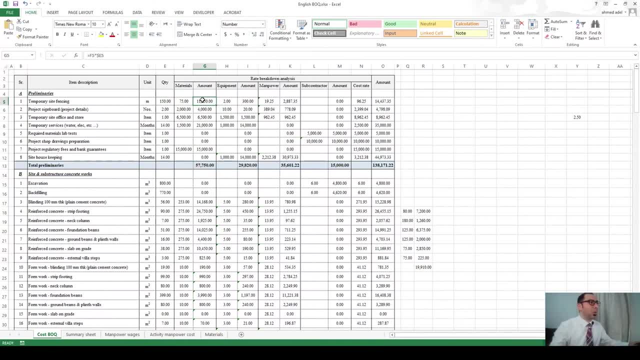 So when the material rate multiplied by the quantity, it will give me the amount of materials required for this item. So if I take a submission here, guys, I understand that for the preliminaries of the project, for example in terms of materials, I need 57,000. 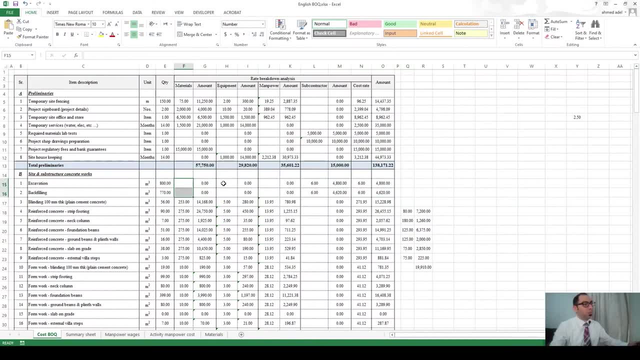 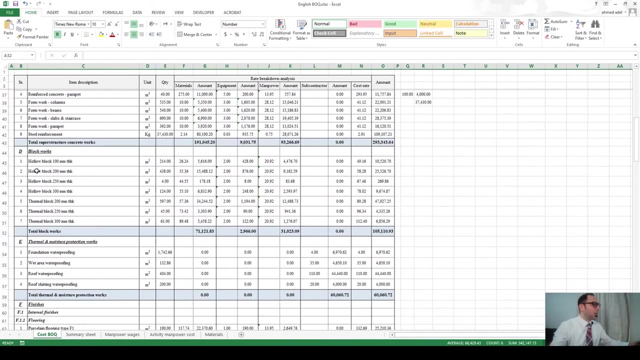 I don't have to help him with anything. Okay, I don't need any means. So if we now, if we go to the BOQ divisions which we have here, prelims, then site works and concrete works, and then we have again superstructure works, block work, thermal and 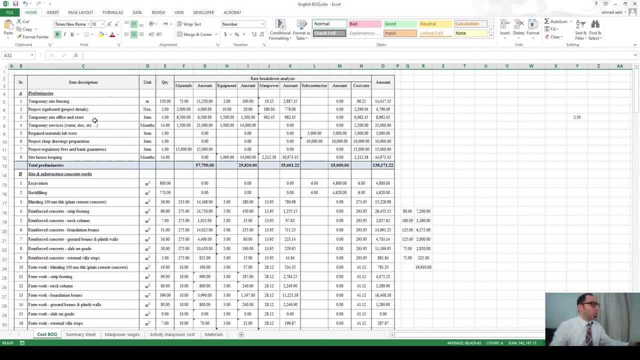 moisture finishes and all of that. Now, if you can see, guys, all these BOQ items, for each and every item I put here how much the material of this item will cost me. So when the material rate multiplied by the quantity, it will give me the amount of materials. 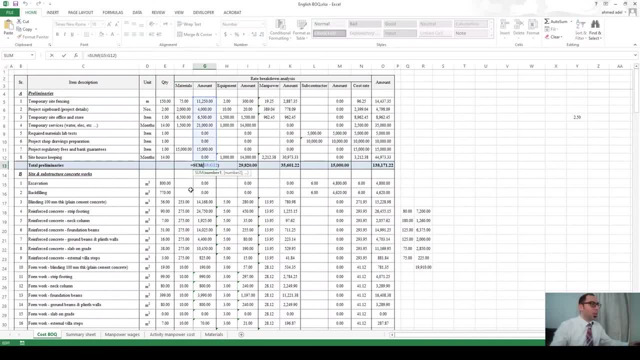 required for this item. So if I take a submission here, guys, I understand that for the preliminaries of the project, for example, in terms of materials I need fifty seven thousand, and equipment I need twenty two thousand, and manpower I need thirty five thousand, and subcontractor I need fifteen. 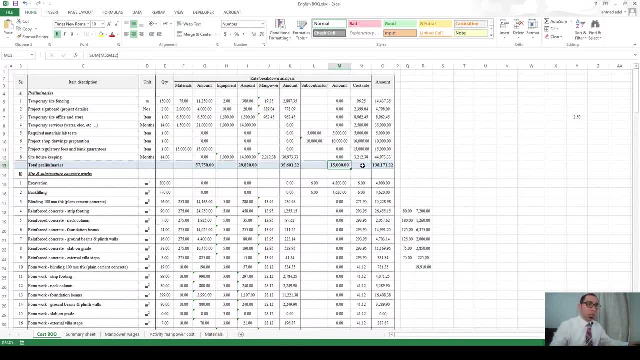 thousand to do some part of the work, Okay. Okay, So the amount of prelims will cost me one hundred thirty eight thousand. And what is the breakdown of the one hundred thirty eight? It is these four numbers. How much is materials, equipment and tools, manpower and subcontractor? 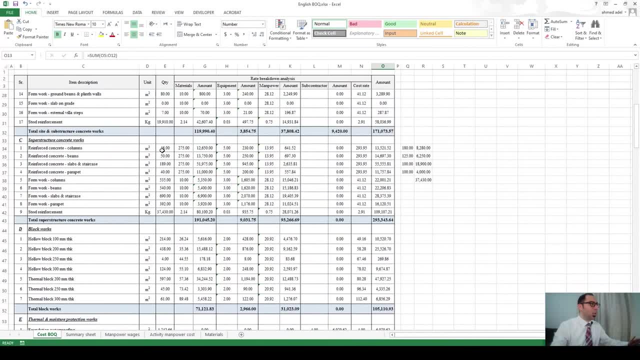 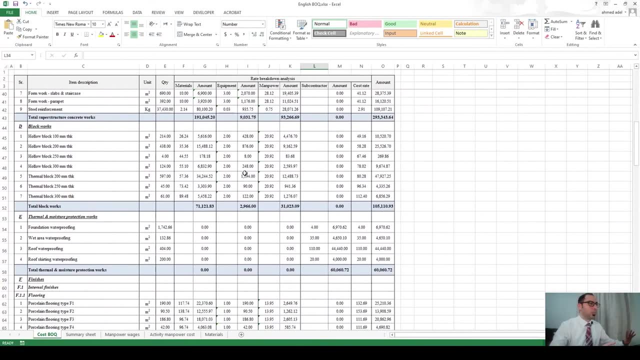 So when you do that for the full project, for each and every item you go, you see how much is the material, how much is the equipment, how much is the manpower, how much is the subcontractor, You do this for all the BOQ divisions. and then when you go to the summary, 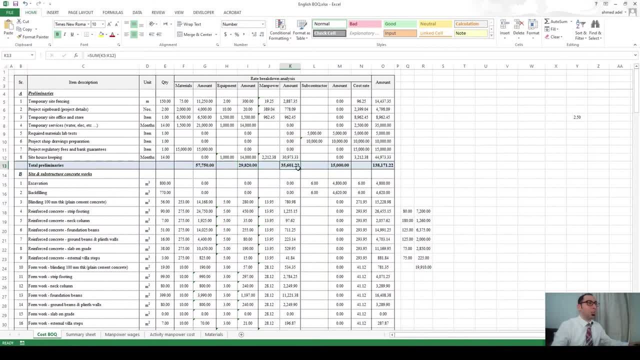 And equipment: I need 22,000.. And manpower: I need 35,000.. And subcontractor: I need 15,000 to do some part of the work. That means that the prelims will cost me 138,000.. 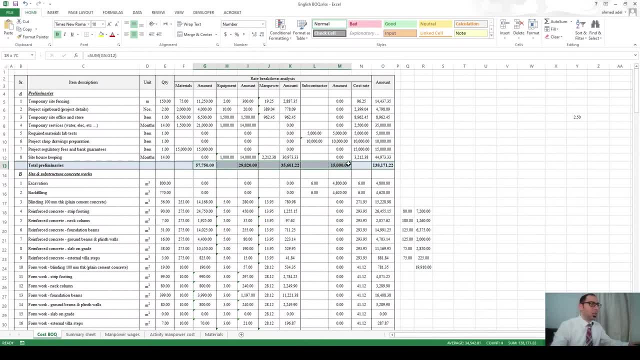 And what is the breakdown of the 138?? It is these four numbers. How much is materials, equipment and tools, manpower and subcontractor. So when you do that for the full project, for each and every item you go, you see how much is the material. 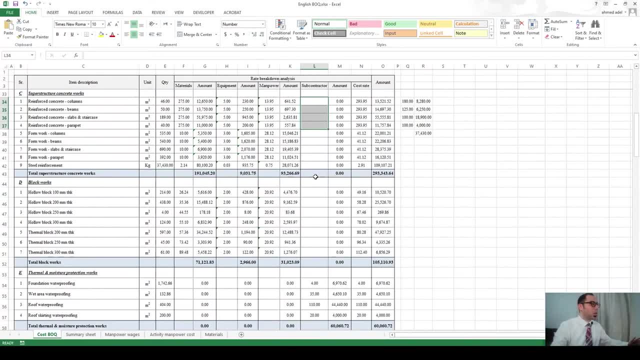 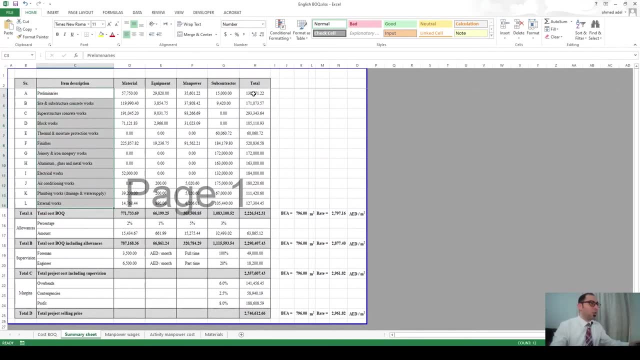 How much is the material, How much is the equipment, How much is the manpower, How much is the subcontractor? You do this for all the BOQ divisions And then, when you go to the summary, instead of having for each BOQ division, instead of having only one total, you will have four totals. 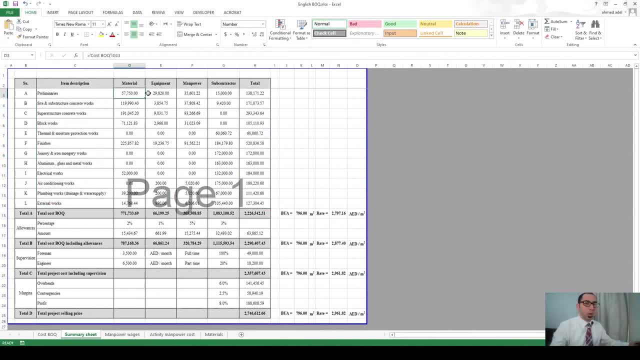 Like for each BOQ division, how much the material will cost, how much the equipment will cost, how much the manpower will cost and how much the subcontractor will cost. So for the full project, For my everything, for the overall project, how much will be the cost of materials? it will be here in this project like 771,000.. 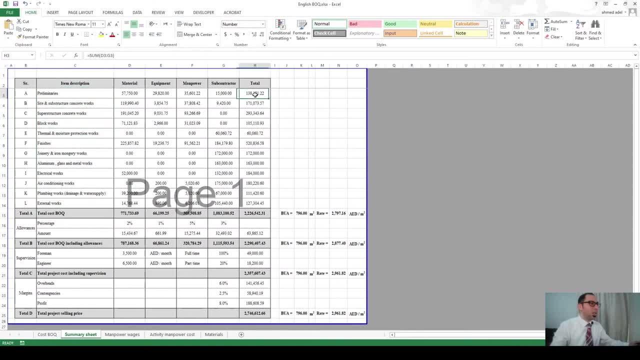 Okay, So instead of having for each BOQ division, and instead of having only one total, you will have four totals, like for each BOQ division: how much the material will cost, how much the equipment will cost, how much the manpower will cost and how much the subcontractor will. 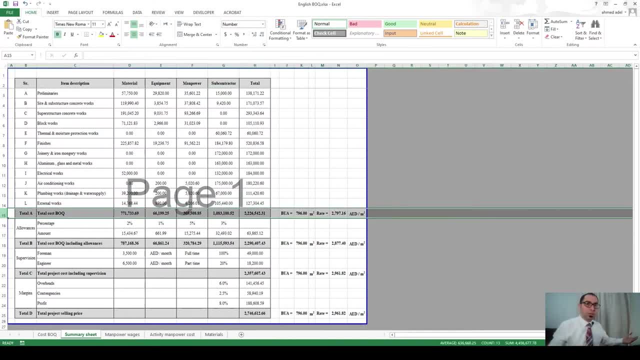 cost. So for the full project, for my everything, for, for the overall project, how much would be the cost of materials- it will be here in this project like seven hundred seventy one thousand- And how much the equipment will cost sixty six thousand and how much the manpower will. 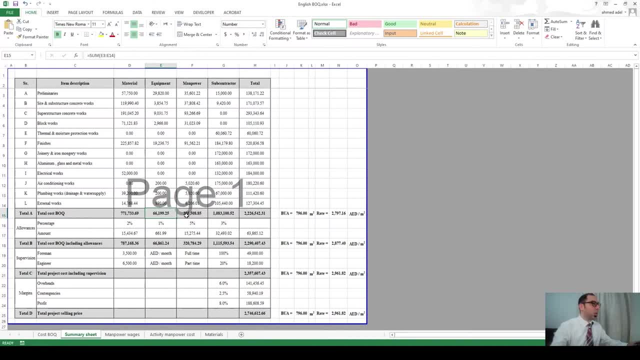 And how much the equipment will cost 66,000.. And how much the manpower will cost- 305,000. And how much the subcontractor will cost about 1 million, And that means that I am subcontracting almost half of the project. 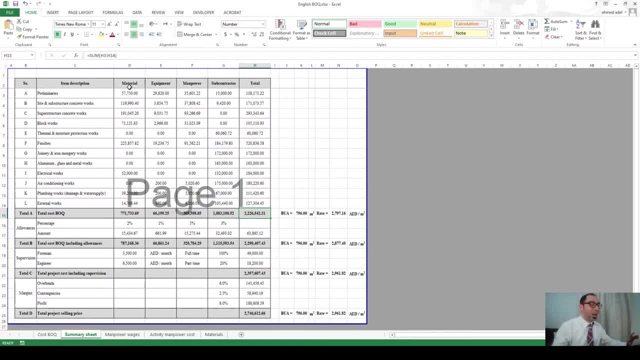 Because the full project cost, in terms of direct cost, Which is material equipment, manpower, subcontractor- These are the direct costs- are the costs that are going directly to be spent on the items or on the works at the site, at the project. 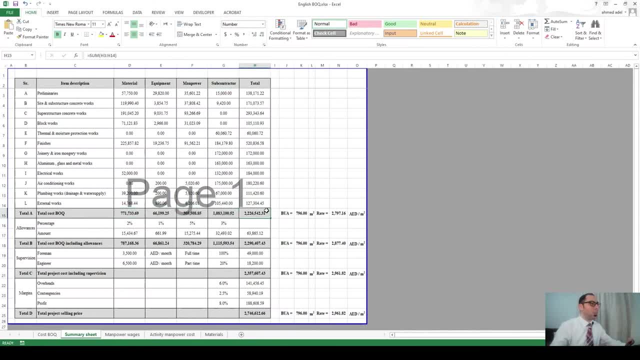 These are the direct costs. So I am having these four numbers And my direct cost is about 2.2 million here. So now I will come to something called allowances. What are the allowances? Now, I have this much. 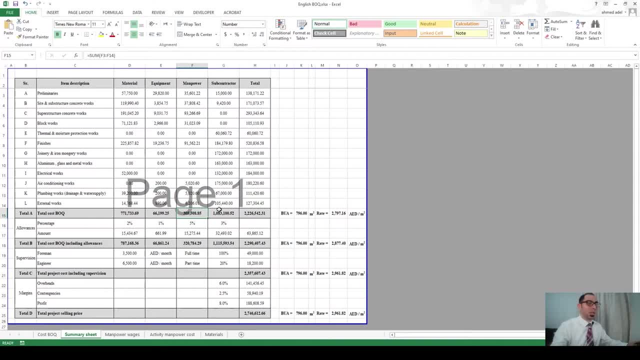 cost three hundred five thousand and how much? the subcontractor will cost about one million And that means that I am subcontracting almost half of the project because the full project cost in terms of direct cost, which is material, equipment, manpower, subcontractor- These are the direct costs, are the costs that are going directly to be spent on the items. 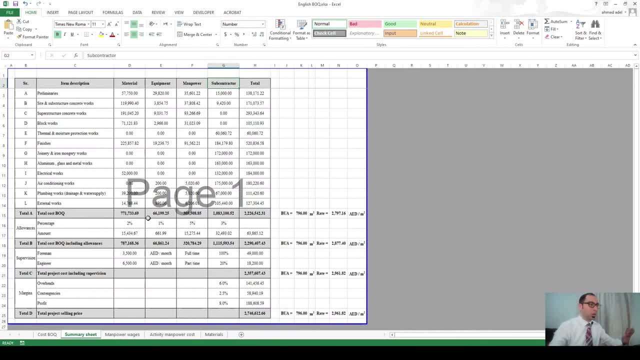 or on the works, at the site, at the project. These are the direct costs. So I'm having these four numbers and my direct cost is about two point two million here. So now I will come to something called allowances. What are the allowances? 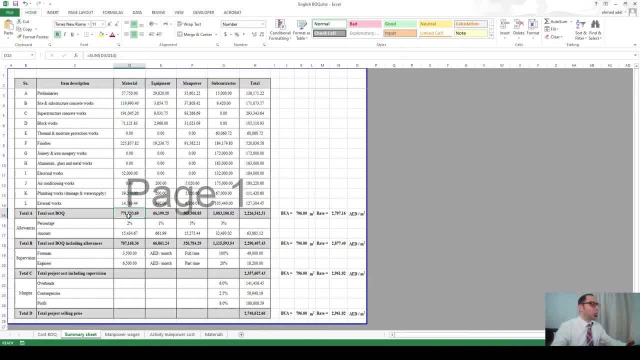 Now I have this much: I have seven hundred seventy thousand materials and actually, in order to derive these numbers, I have like assumed that the wastage, and I have assumed and I have Considered so many factors. but again here I am saying that, OK, maybe these materials, 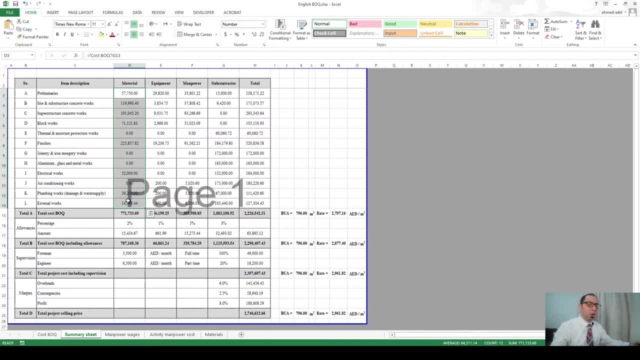 it requires some, let's say, shifting or some some kind of of of of service that I have not considered here. So I'll allow for two percent of the seven hundred seventy more as an allowance for something guys like for the material shifting, If I haven't. 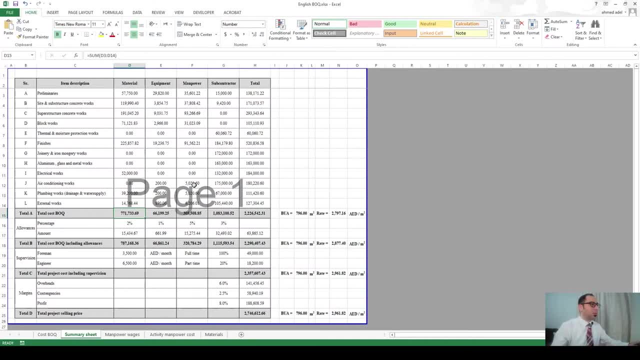 Like I counted for the shifting or something like that. Now let's talk about, for example, the manpower I have here, manpower of three hundred five thousand, So I have not considered any idle manpower. or sometimes I'll send two, three laborers or five laborers or ten laborers to the project and they will not have anything to do due. 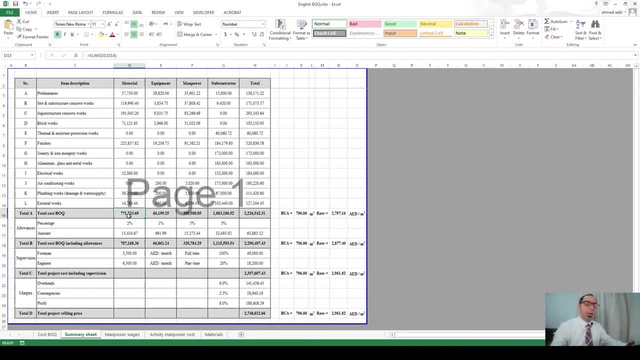 I have 760.. I have 770,000 materials And actually, in order to derive these numbers, I have assumed the wastage And I have assumed and I have considered so many factors. But again here I am saying that, okay, maybe these materials it requires some, let's say, shifting or some kind of service that I have not considered here. 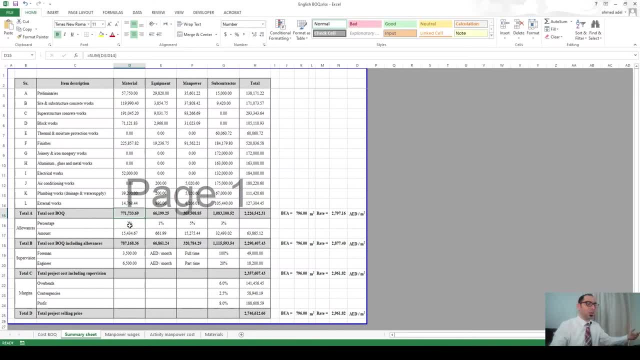 So I'll allow for 2% Of the 770,000 more as an allowance for something guys Like for the material shifting, if I haven't like accounted for the shifting or something like that. Now let's talk about, for example, the manpower. 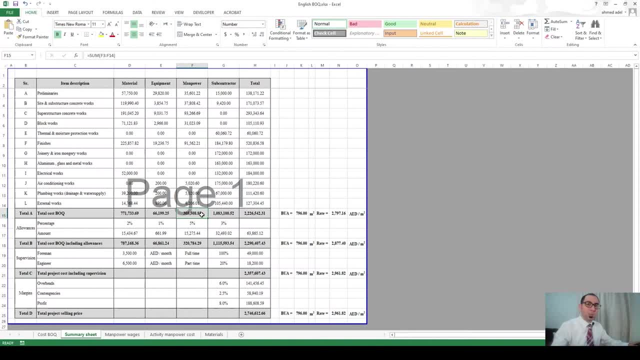 I have here manpower of 305,000. So I have not considered any idle manpower. or sometimes I'll send 2,, 3 labors or 5 labors or 10 labors to the project And they will not. They will not have anything to do due to any restrictions or anything happening at the site. 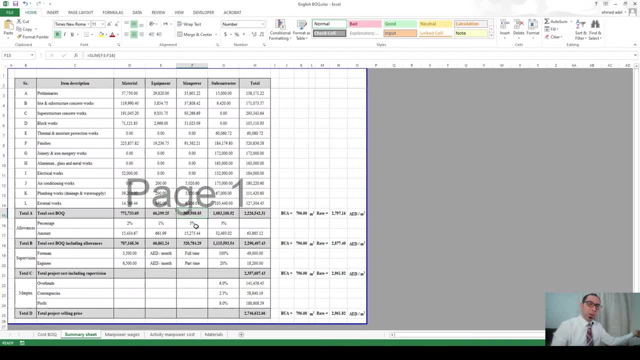 So in that case I am losing in that day because I will pay the labors in that day and they will not work. So I am just assuming here that or I am allowing for 5% extra on top of what I have already considered as money that I will pay to the manpower due to idle times or all these things. 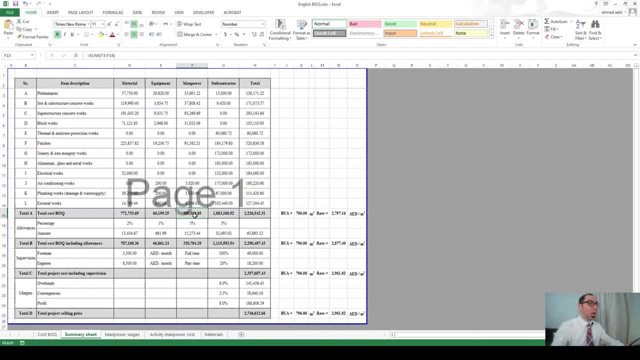 to any restrictions or anything happening at the site. So in that case I am losing in that day because I will pay, I will pay the laborers in that day and they will not work. So I am Just assuming here that or I am allowing for five percent extra on top of what I have already. 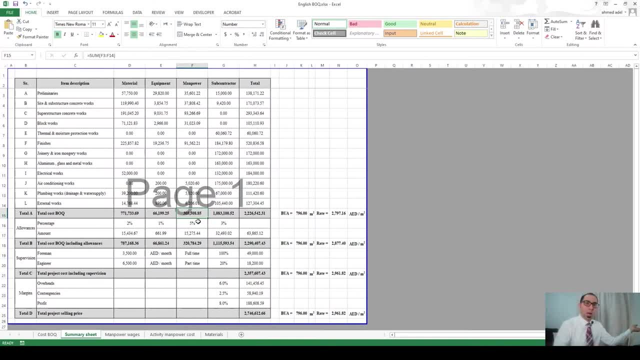 considered as money that I will pay to the manpower due to idle times or all these things. for subcontractors, For example, I am adding to whatever cost I am arriving based on the subcontractor quotations. I'm adding three percent here or I am allowing for three percent more for any services that. 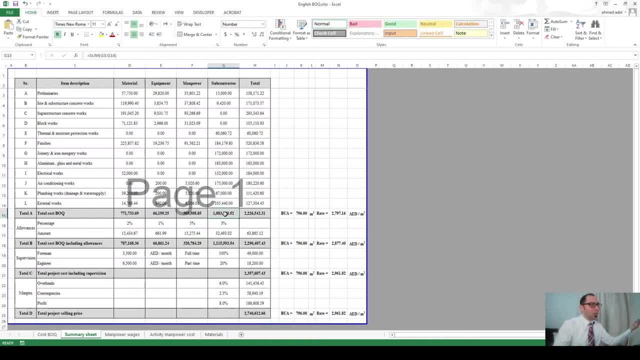 For subcontractors, for example, I am adding 2%. So whatever cost I am arriving based on the subcontractor quotations, I am adding 3% here, or I am allowing for 3% more for any services that will be required by me as a main contractor towards these subcontractors to help them execute or continue their job. 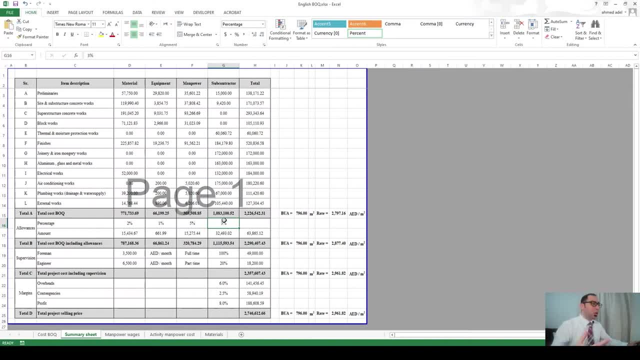 Guys, that's why it is called cost estimation. I am not calculating anything here. I am estimating, And even it's me who estimated this project. If I want to estimate this project one more time, I will end up with different numbers. 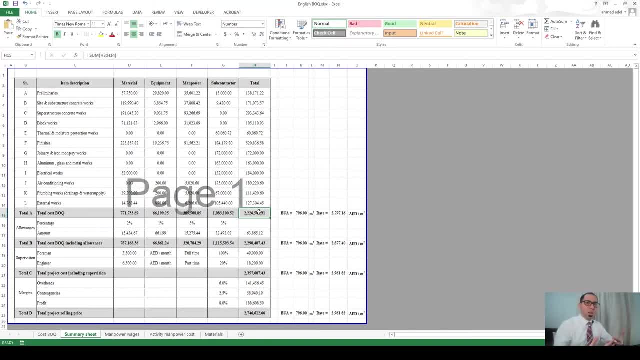 The numbers will not be the same. Maybe the difference will be very slight, but still So. imagine if two people are doing cost estimation for the same project. Definitely or 100% sure they will not arrive the same exact figure because each of these two estimators is having his assumptions. 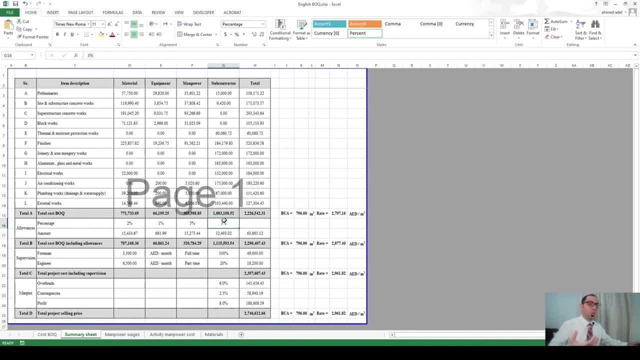 be required by me, as a main contractor towards these subcontractors, to help them execute or continue their job. guys, that's why it is called cost estimation. i am not calculating anything here. i am estimating, and even it's me who estimated this project. if i want to estimate this project, 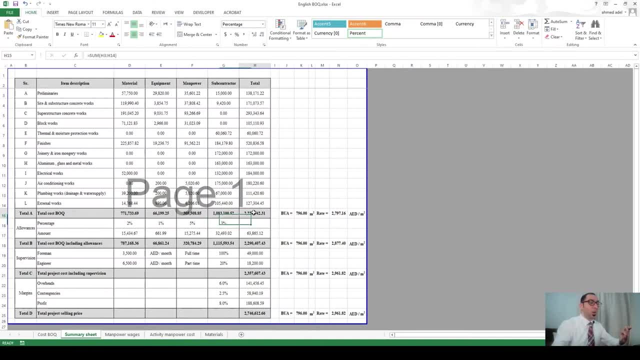 one more time. i'll end up with different numbers. the numbers will not be same, maybe the difference will be very slight, but still so. imagine if two people are doing cost estimation for the same project. definitely, or 100, sure they will not arrive the same exact figure, because each of these 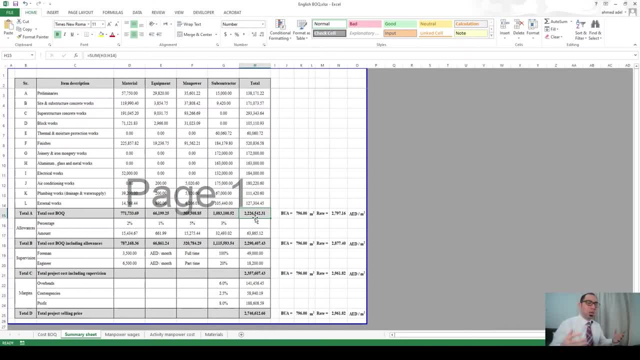 two estimators, is having his assumptions, he is having his price list, he is having some understanding about the labor productivity. i might say that one mason will do 10 meters per day and some other estimator will say no one mason will do minimum 12 meters per day. so our prices will be different, but we will be. 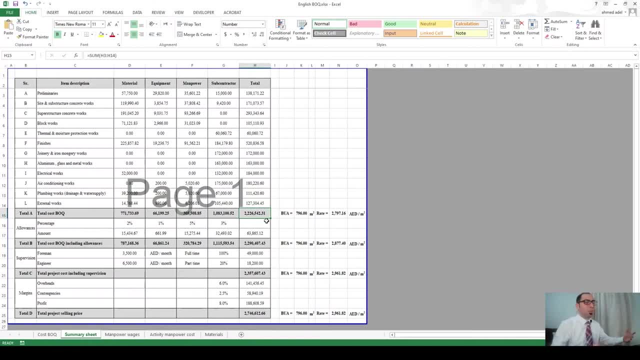 like arriving something around this or near, like more or less. but in the end our both estimates are not wrong. it's both correct. but what i want to tell you, you will say: you just go like that and you throw a three percent on top of this, or you go here and you throw a five percent on top. 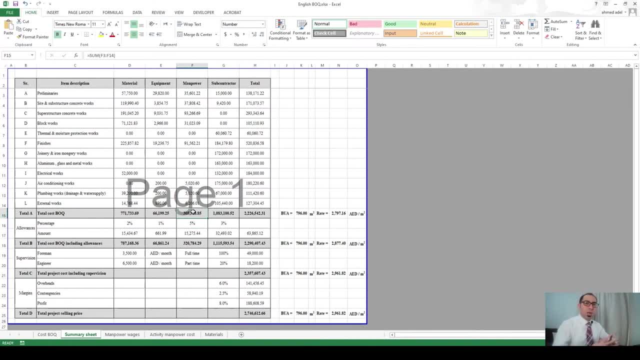 of this, guys. this is that's why it is called the estimation. we are not calculating, we are not accounting, we are estimating. i am estimated. that's why it is called cost estimation, guys. okay, so, after i have, uh, made these allowances, these percentages on top of each, 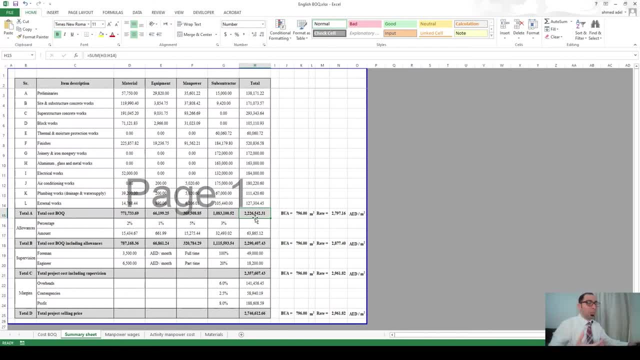 He is having his price list. He is having some understanding about the labor productivity. I might say that one mason will do 10 meters per day and some other estimator will say no one mason will do minimum 12 meters per day. 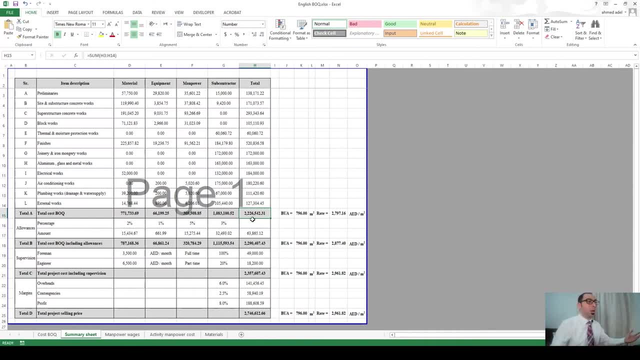 So our prices will be different, but we will be like arriving something around this or near, like more or less. But in the end our both estimates are not wrong. It's both correct. But what I want to tell you, you will say: you just go like that. 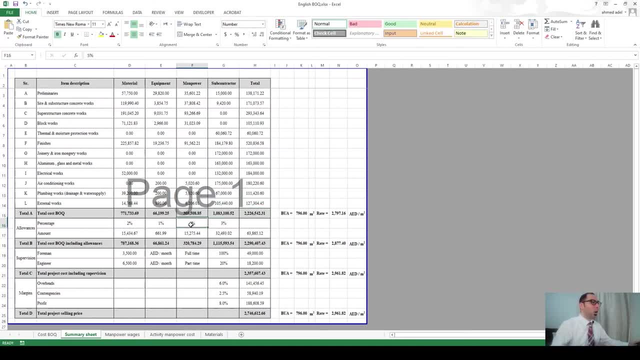 And you say, okay, I am going to do this. You throw a 3% on top of this, or you go here and you throw a 5% on top of this. Guys, this is that's why it is called the estimation. 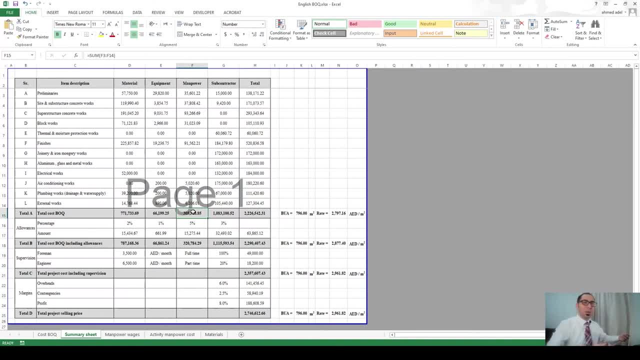 We are not calculating, We are not accounting, We are estimating. I am estimating. That's why it is called cost estimation, guys. Okay, So after I have made these allowances, these percentages on top of each one of them, So I am getting here total cost, BOQ, including allowances. 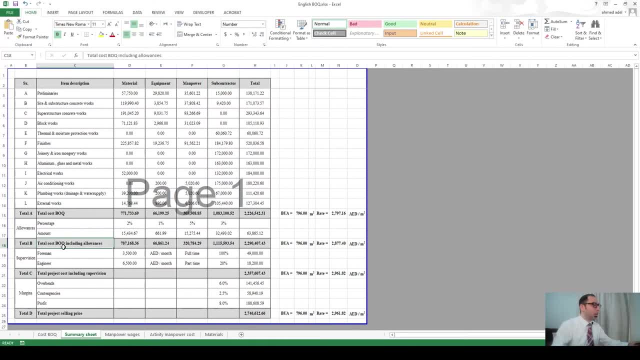 one of them. so i am getting here. total cost, boq including allowances, the 770 will be 787. see guys, it is very slight differences, but it might cover me in case something happens that i have not for now. let's come to the site supervision. i've noticed that in in my boq here there was no any. 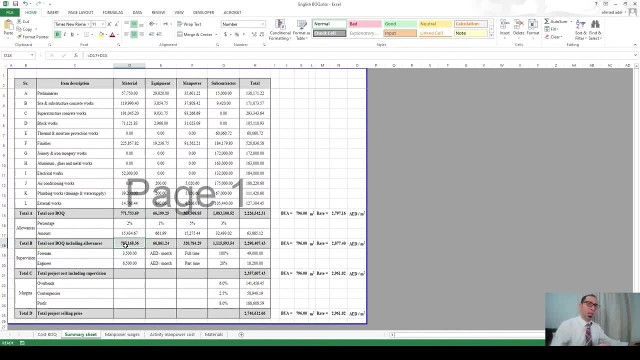 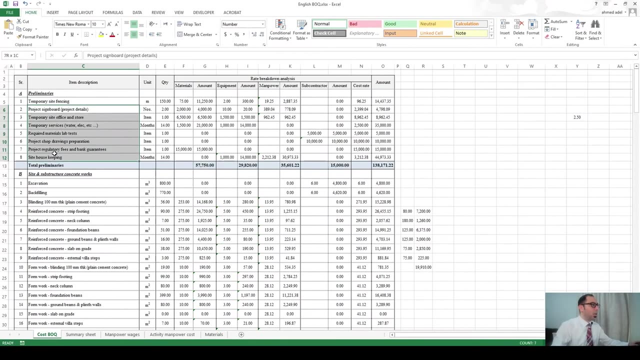 The $700.. 70 will be $787.. See, guys, it is very slight differences, but it might cover me in case something happens that I have not accounted for. Now let's come to the site supervision. I have noticed that in my BOQ here there was no any item in the preliminaries for the site supervision. 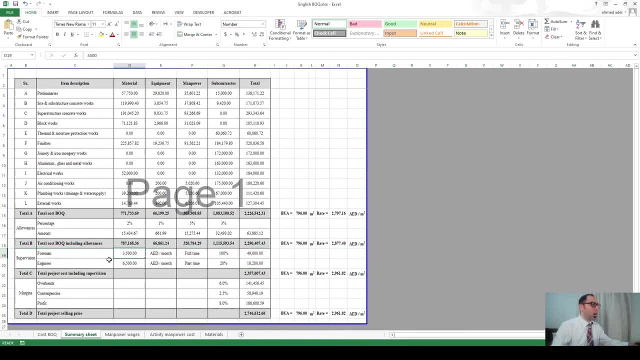 So what I did? I came here and I assumed that there will be a foreman and his salary is this much, So he will be at the site 100% of the time. He is there full time. So his salary multiplied by the duration of the project, and this will give me how much this foreman will cost me. 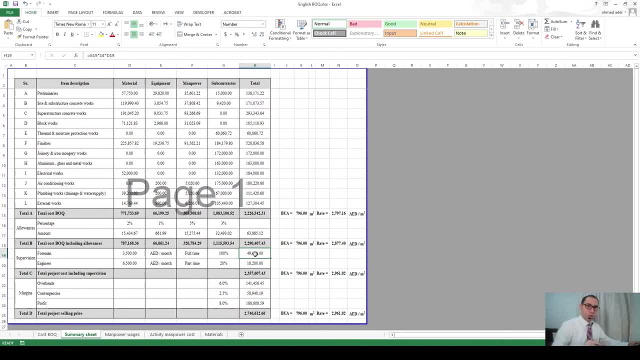 And this cost has to be loaded on this project because this foreman will work full time on this project. But if I need some help from the technical engineer who is sitting in my office, he will do some shop drawing or he will do something to serve the execution of this project. 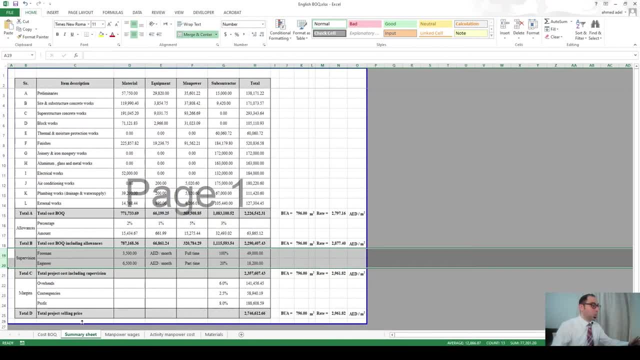 item in the in the preliminaries for the site supervision. so what i did? i came here and i assumed that there will be a foreman and his salary is this much, so he will be at the site hundred percent of the time. he is there full time. so his salary multiplied by the duration. 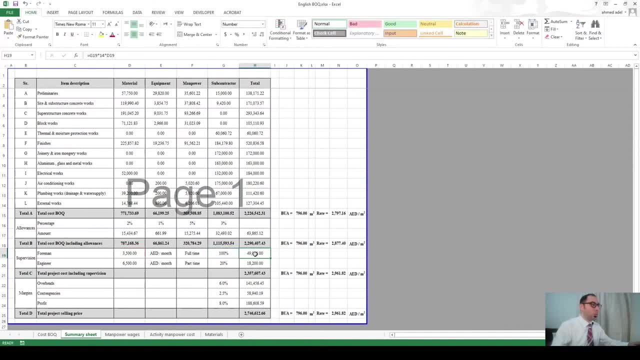 of the project and this will give me how much this foreman will cost me. and this cost has to be loaded on this project because this foreman will work full time on this project. but if i need some help from the technical engineer who is sitting in my office, he will do some shop drawing or he will do something to serve. 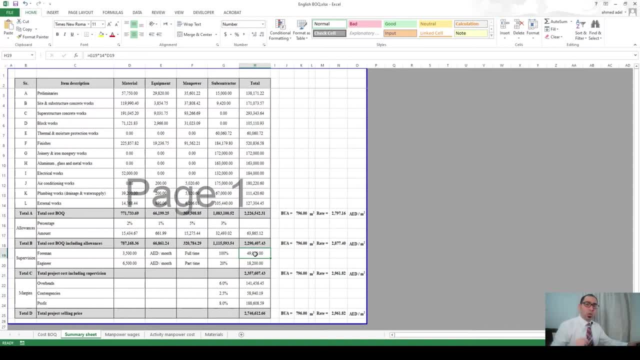 the execution of this project. i cannot charge his full salary to this project only because he is not working only on this project. he is working maybe on this project and two, three, four other similar projects. he is working on them at the same time. so these two, the foreman and the 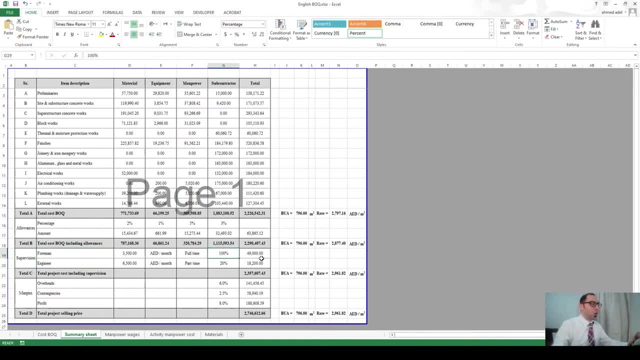 engineer- the former, for example. here i am assuming that he will work full time on this project, and i am assuming that the engineer will have five similar projects similar to this one. he will be supervising all of them at the same time, but each one of these five projects will have its own. 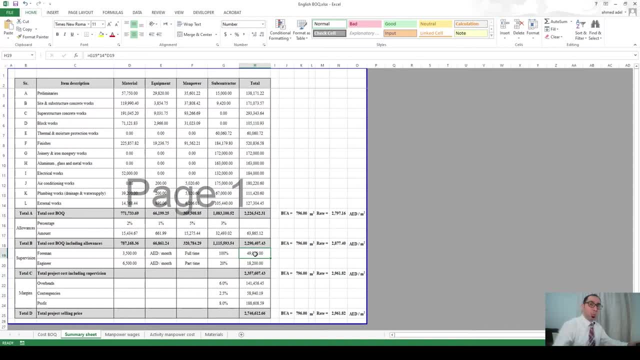 I cannot charge his full salary to this project only because he is not working only on this project. He is working maybe on this project and two, three, four other similar projects. He is working on them at the same time. So these two, the foreman and the engineer, the foreman, for example, here I am assuming that he will work full time on this project. 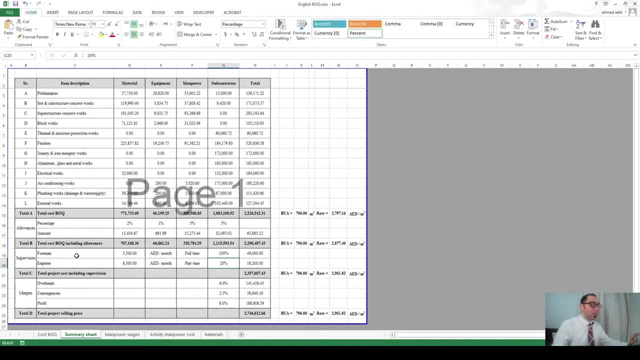 And I am assuming that the engineer will have five similar projects similar to this one. He will be Supervising all of them at the same time, But each one of these five projects will have its own foreman, who will be there full time. 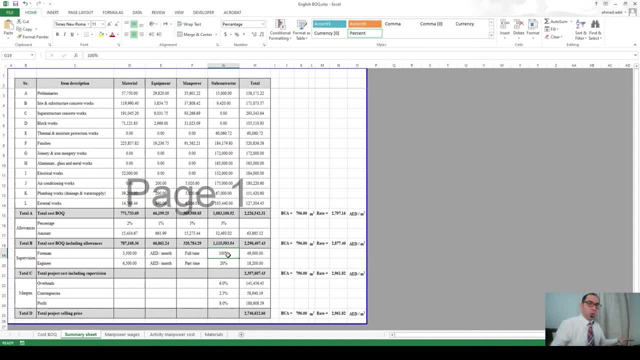 So for the five projects, in each project a foreman will be there full time and the engineer will be like one-fifth of his time in each of these projects. He will supervise five projects at the same time with the help of a foreman in each project, who will be there full time. 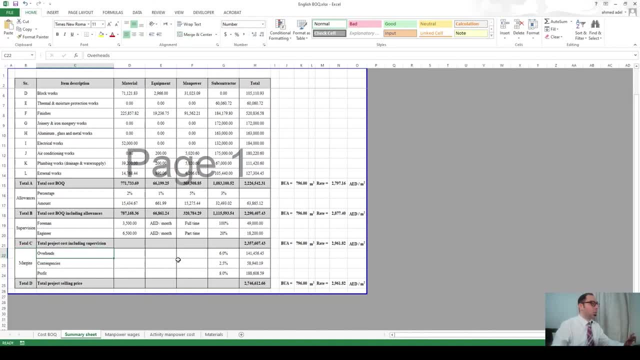 Now let's come and talk about the margins. The margins: here there is something called the overheads guys, which I just told you Now, the rent of my office, or the salary of the accountant who is working in my head office, okay, or the electricity and telephone and all these utility bills for my head office. 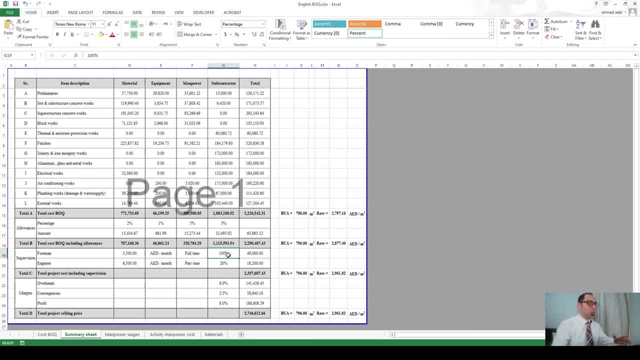 foreman who will be there full time. so for the five projects in each project, a foreman will be there full time and the engineer will be like one fifth of his time in each of these projects. he will supervise five projects at the same time with the help of a foreman in each project, who will be there full time. 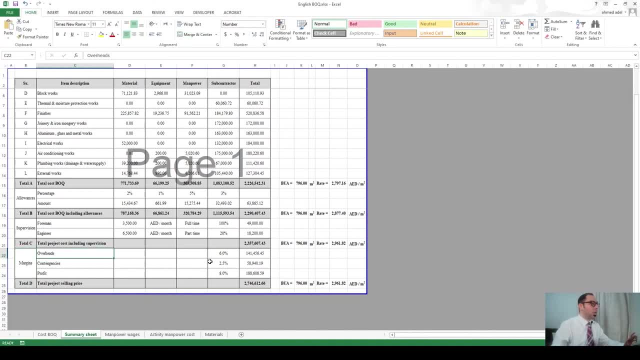 now let's come and talk about the margins. the margins: here there is something called the overheads, guys, which i just told you now: the rent of my office, or the salary of the accountant who is working in my head office, okay, or the electricity and telephone and all these utility bills for my head office. which project, which project will bear these? 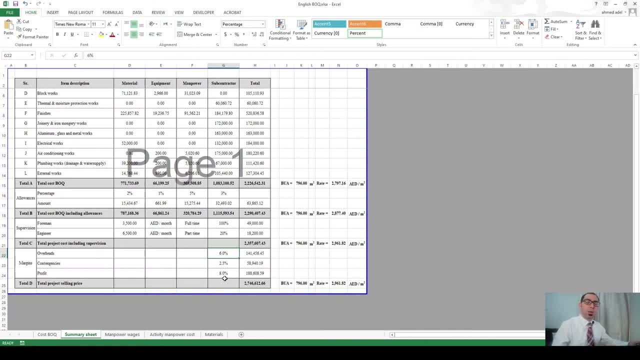 Which project? which project will bear these costs? I have five projects or six. All of them, guys, should bear the cost of having a head office or having something that indirectly affecting the cost of my project. So how to calculate this? 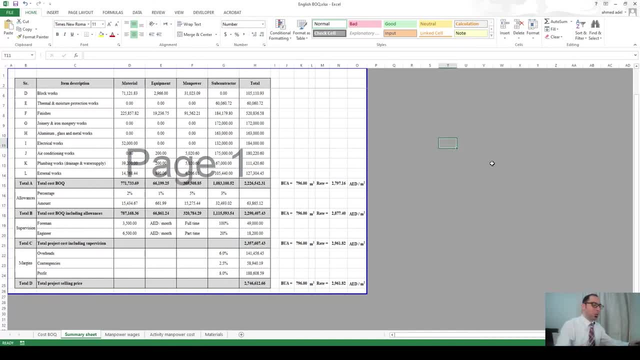 Let's say that I have a company, I am a main contractor and I have four projects. The first one is $2,500,000. And the other. the next one is $3,000,000. And I have a project. 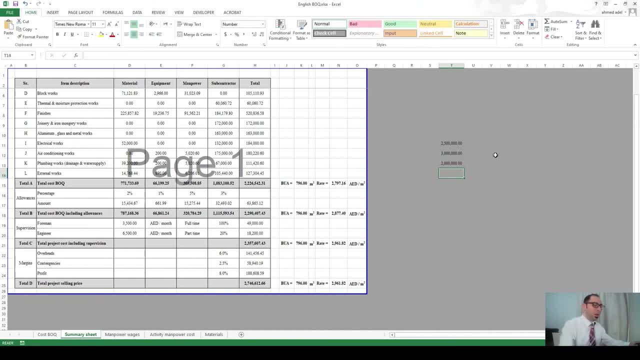 I have a project of $2,000,000 and I have another project of $3,500,000. So my total projects is $11,000,000.. Okay, And let's say that I have a monthly spend of, let's say, $50,000 per month. 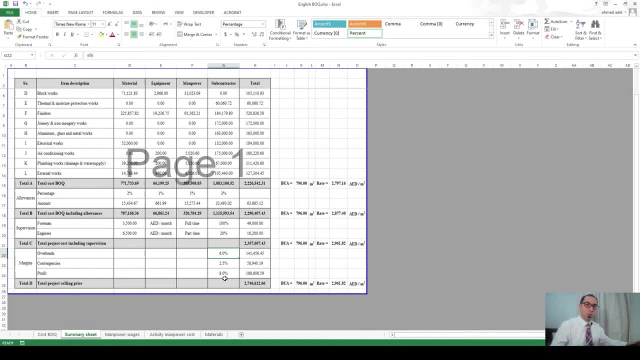 costs. i have five projects or six projects. all of them guys should bear the cost of having a head office or having something that indirectly affecting the cost of my project. so how to calculate this? let's say that i have, i have a company, i am a main contractor and i have four projects. the first one is two, two million five hundred. 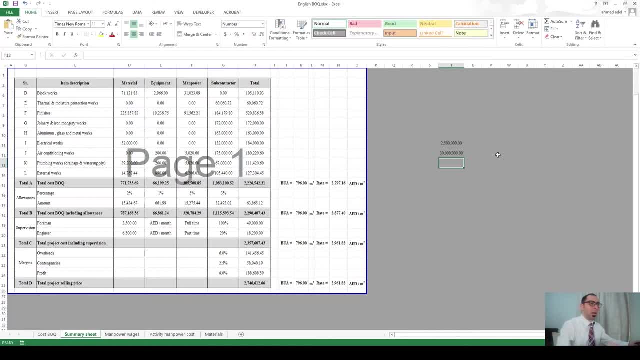 thousand and the other. the next one is three million and i have a project of two million and i have another project of three million five hundred thousand. so my total projects is a 11 million. okay, and let's say that i have a monthly spend of, let's say, 50 000 per month. 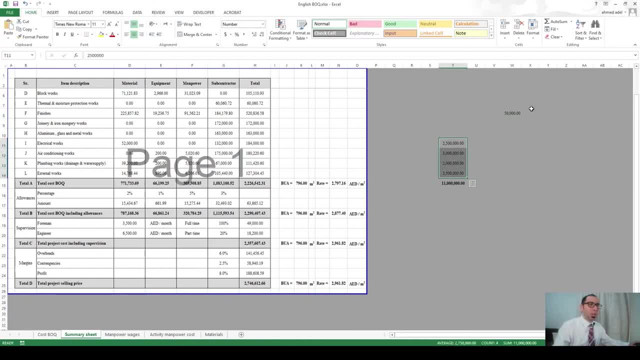 okay, and the duration of each of these projects is 14 months. so as i am executing these four projects, or these four jobs, as at the site, as i am executing them at the site, my office is running, and how much i am paying, i am paying 50 000 into 14. so in the 14 month that i will execute, 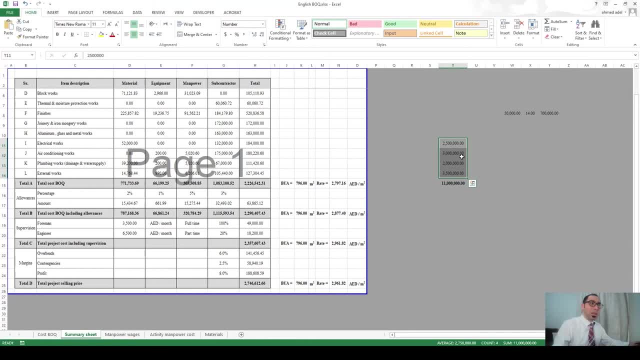 these projects i'll be spending indirectly an amount of 700 000. so this 700 000, these projects should should bear it, should bear it, and which of them will bear more of the 700 000? i have to understand the percentage of each of them. like the first one is 23. 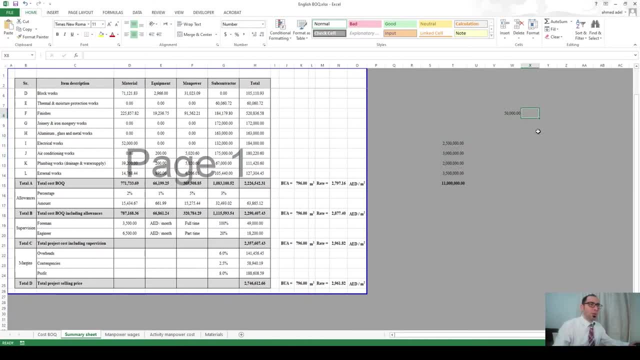 Okay, And the duration of each of these projects is 14 months. So, as I am executing these four projects, or these four jobs, At the site, as I am executing them at the site, my office is running And how much I am paying. 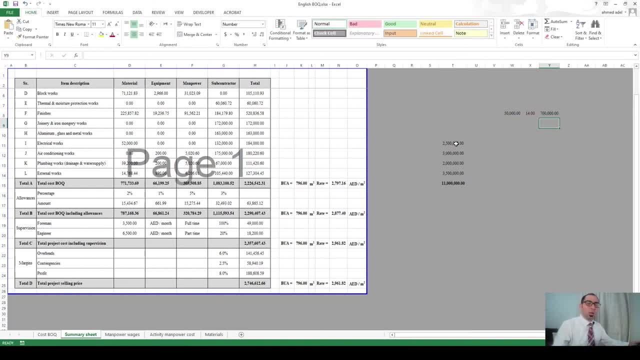 I am paying $50,000 into 14.. So in the 14 months that I will execute these projects, I will be spending indirectly an amount of $700,000.. So this $700,000, these projects should bear it. 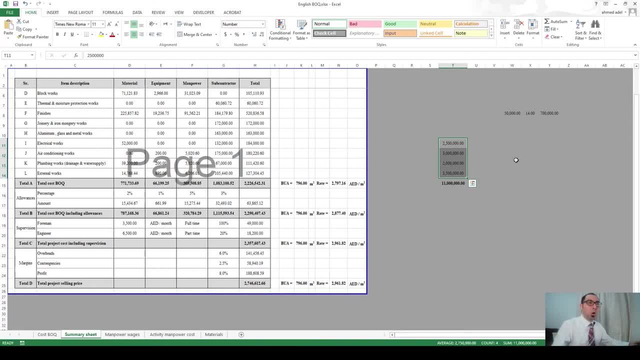 Should bear it And which of them will bear more of the $700,000?? I have two. Understand. the percentage of each of them, Like the first one, is 23%, Here Like now, in terms of value, let's say. 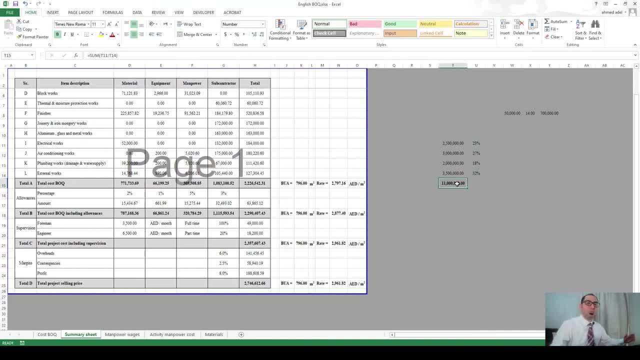 Okay, This project is 23% of my total company work. This project is 27%. This project is 18%. This project is 32%. So this is the biggest project. He will bear the biggest amount or the biggest portion from this indirect cost. 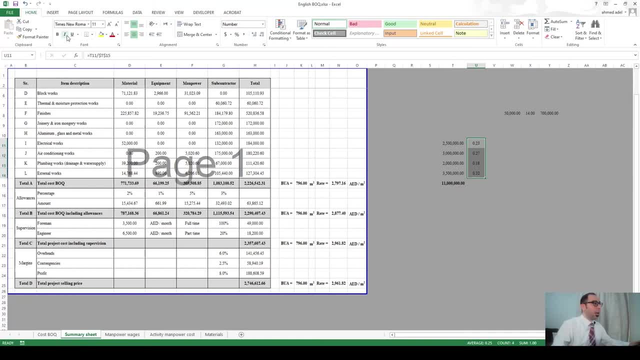 粒 percent here, like now. in terms of value, let's say: okay, this project is 23 percent of my total company work. this project is 27 percent, this project is 18, this project is 32. so this is the biggest project. he will bear the biggest amount or the biggest portion from this indirect cost or 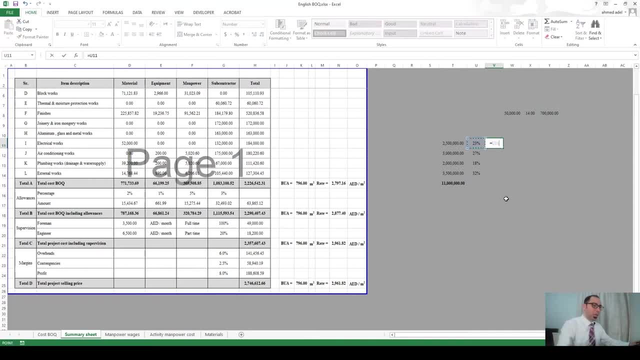 these overheads. so if i come here and i'll say equal to the percentage into this, so this project should bear as an overhead an amount of 159, 159 in 14 month. so if you can see, here for this project i have considered a percentage from the cost that i calculated. 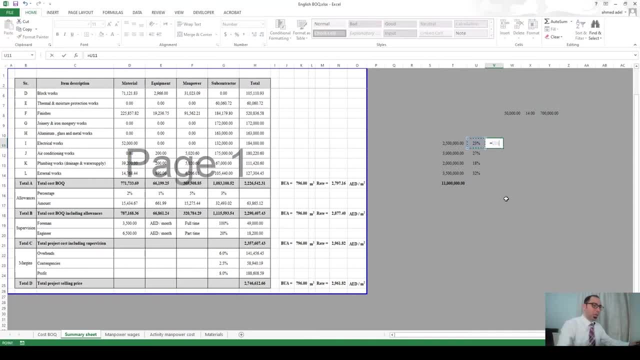 Or these, These overheads. So if I come here and I'll say equal to the percentage into this, So this project should bear as an overhead an amount of $159,000.. $159,000 in 14 months. So if you can see, here for this project I have considered a percentage from the cost that I calculated for this project to cover me here. 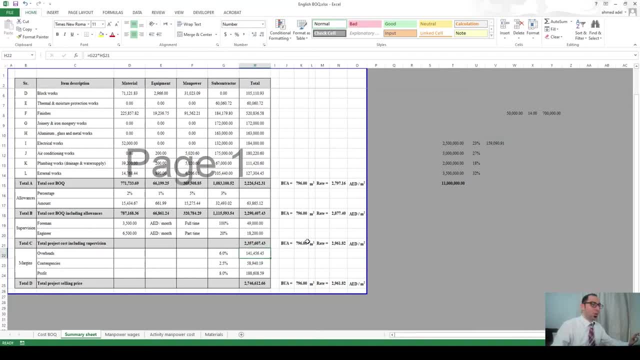 If you can see, here I am considering, I am considering something like $141,000.. And here you see, guys, a project similar to this one, Because you see $2,000, almost $400,000 or $2,700,000. 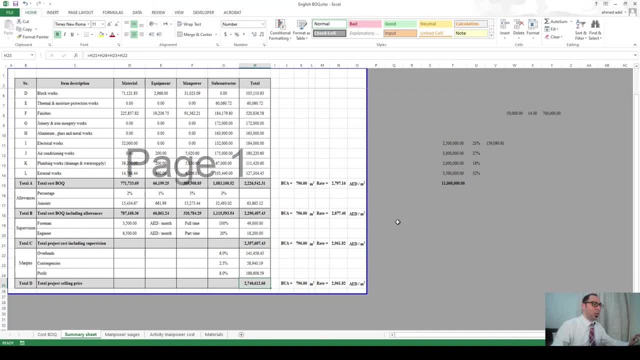 And this project is sorry, $2,000,000.. $2,700,000.. And this project is $2,500,000.. Almost the same guys. So I am assuming a percentage of the cost that will cover this amount. 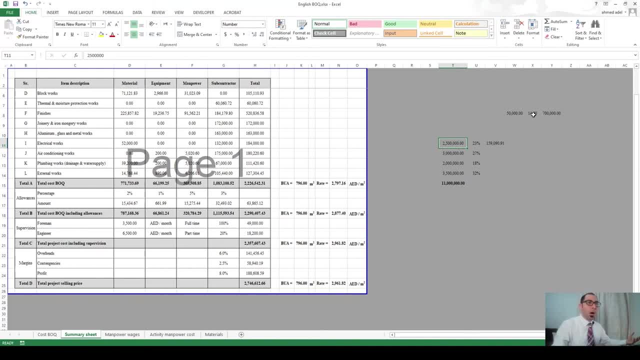 Because this project should bear from my 14-month expenses. It should carry, or I should load, Okay- An amount of $159,000 in here to pay for whatever I am doing in my head office to serve my jobs or my projects to run. 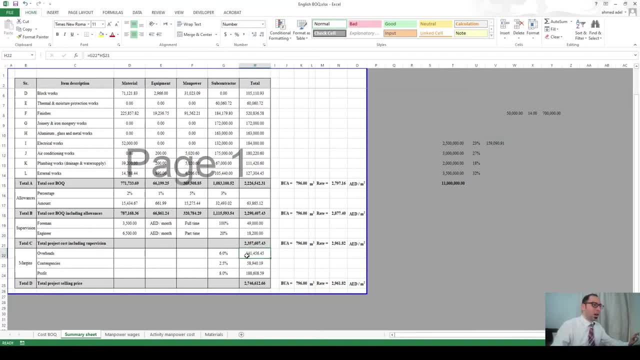 for this project to cover me here, if you can see, here i'm, i'm, i'm, i'm considering something like 141, and here you see, guys, a project similar to this one, because you see 2000, almost 400 or 2700, and this project is, is sorry, 2 million, 2 million, 700, and this project 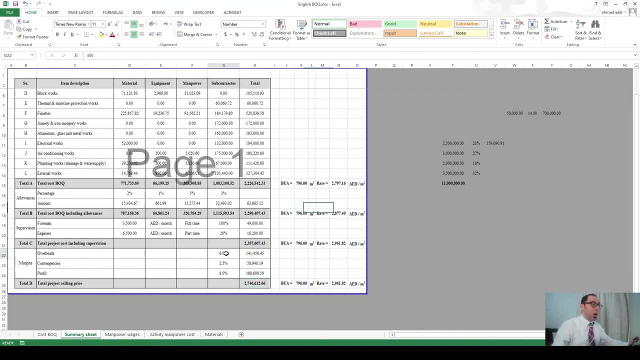 is 2 million 500- almost same guys. so i am assuming a percentage of the cost that will cover this amount, because this project should bear from my 14 month expenses it should carry. or i should load an amount of 159 000 in here to pay for whatever i am doing in my head office to serve my 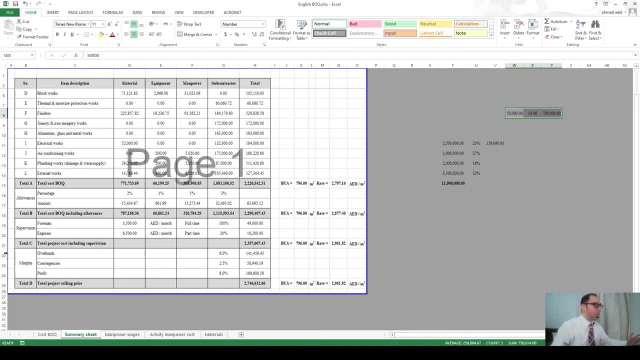 jobs or my projects to run, and this is the definition of overheads and this is how we calculate the overheads. usually nobody is doing that, guys, but i did this just to show you how it is done, but sometimes, or most of the time, they calculate the overheads something from 6 to 12. 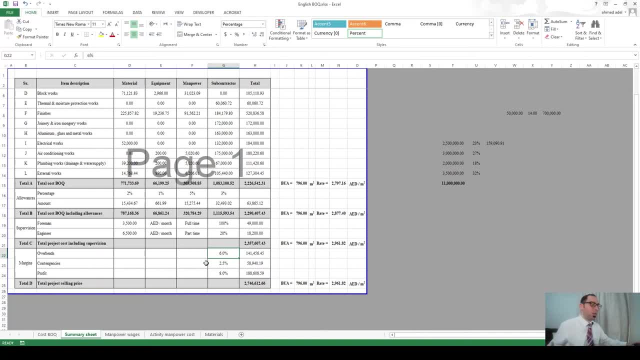 percent. it depends on how many engineers you have in your head office, how many draft men, how many office boys, accountants and secretaries and all these people who are not directly loaded on one of your company projects. now, contingencies, contingencies are the things that i have not. 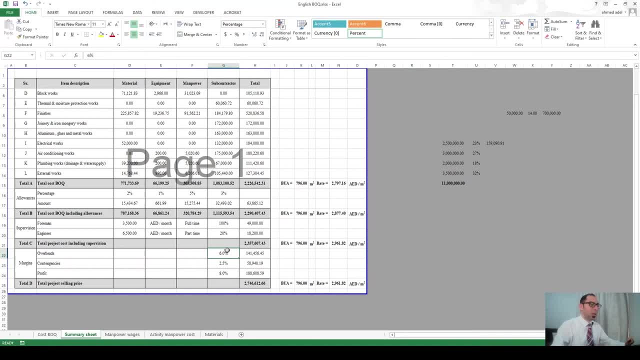 And this is the definition of overheads And this is how we calculate the overheads. Usually nobody is doing that, guys, But I did this just to show you how it is done, But sometimes, or most of the time, they calculate the overheads something from 6% to 12%. 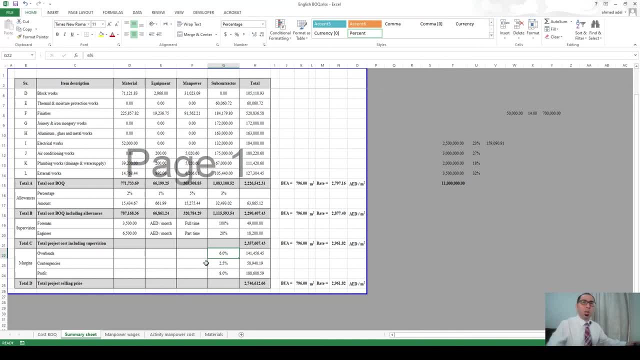 It depends on how many engineers you have in your head office, How many draft men, How many, How many office boys, accountants and secretaries and all these people who are not directly loaded on one of your company projects. Now contingencies. 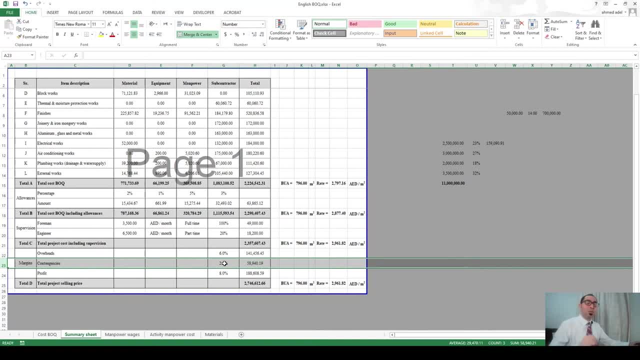 Contingencies are the things that I have not thought of. Like, if there is any risk that I have, because, guys, the risk is unplanned event, Like it's something that you cannot predict. So if I can predict something, If you remember, guys, when I spoke to you about the allowances, I am predicting that my manpower will be sometimes idle. 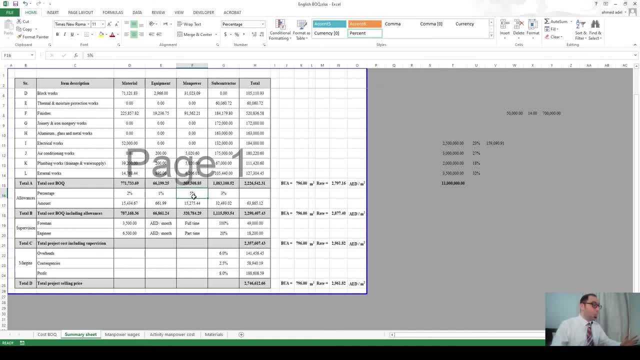 That's why I put here 5%. But the contingency? what is the difference between the contingency and the allowance? Allowance is something that I am assuming or I am predicting. I am seeing it coming, So that's why I have allowed for 5% here. 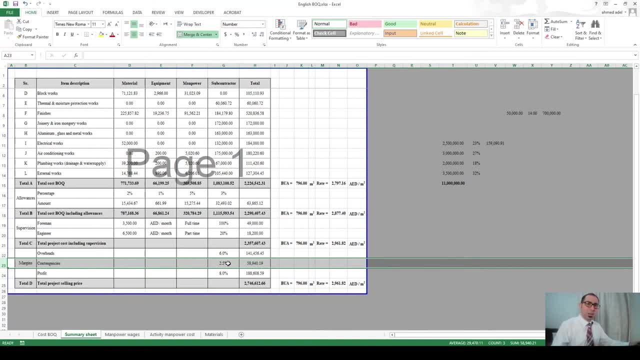 thought of, like, if there is any risk that i have, because the guys the risk is unplanned event, like it's something that you cannot predict. so if i can predict something, if you, if you remember, guys, when i spoke to you about the allowances, i am predicting that my 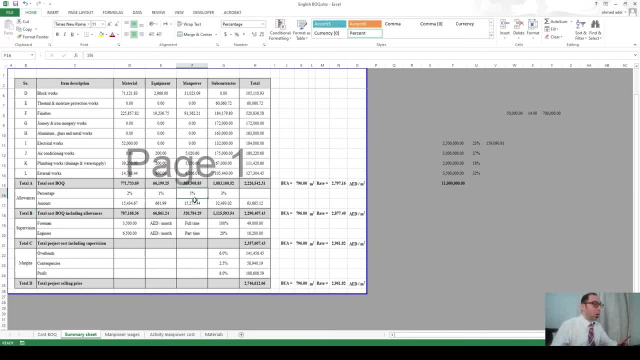 manpower will be sometimes idle. that's why i put here five percent. but the contingency? what is the difference between the contingency and the allowance? allowance is something that i am assuming or i am predicting. i am seeing it coming, so that's why i've allowed for five percent here. 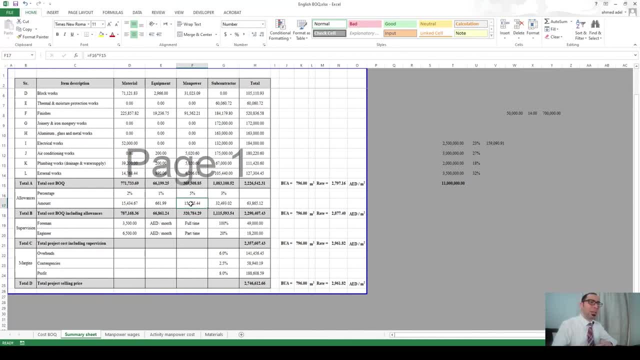 but what about the, the events that i am not foreseeing, the events that i don't know they will come or no? i'm keeping here 2.5 percent, like, as, let's say, risk margin or for whatever things that i have not allowed for or something i have missed. 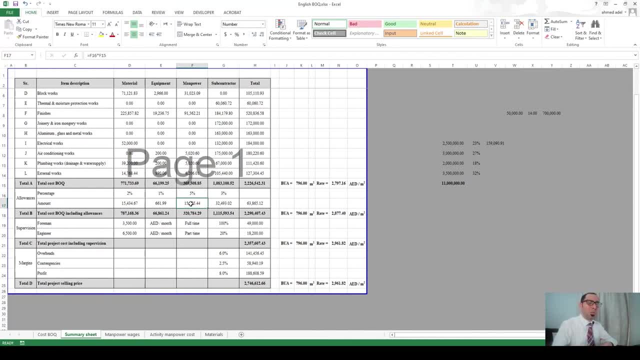 But what about the events that I am not foreseeing, The events that I don't know they will come or no? I am keeping here 2.5%, like, as, let's say, risk margin or for whatever things that I have not allowed for or something I have missed here and there. 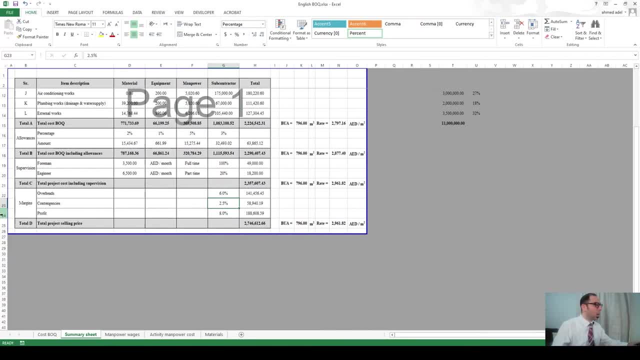 Because, as I told you guys, it's just an estimation. Okay, what about the profit? I am assuming here 8% from this cost as a profit. So, overheads plus contingencies plus profit, This is my overhead, This is my overall margin, which is 16.5.. 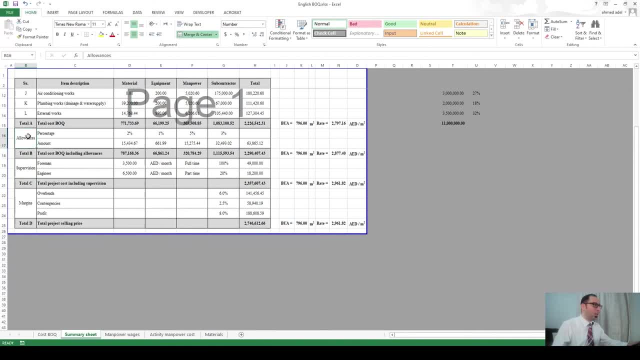 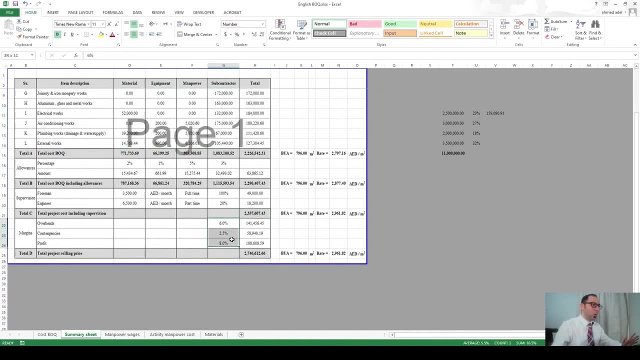 So when this cost- okay, including the supervision, the allowances and everything else that I have priced inside- if my cost is 2.3, when I add the 16.5%, I will arrive a selling price. This is the price that I will give to my client. 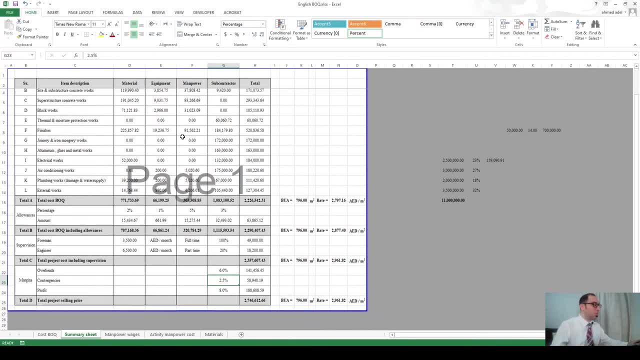 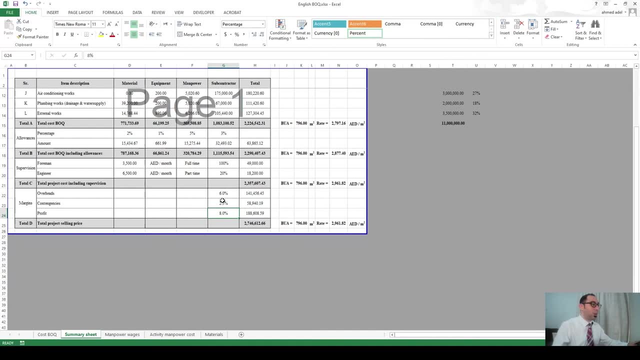 here and there, because, as i told you guys, it's just an estimation. okay, what about the profit? i am assuming here eight percent from this cost as a profit, so overheads plus contingencies, plus profit. this profit is going to be 8 percent from this cost as a profit, so overheads plus contingencies. 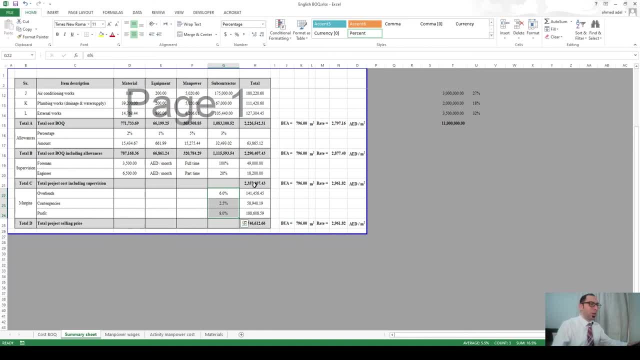 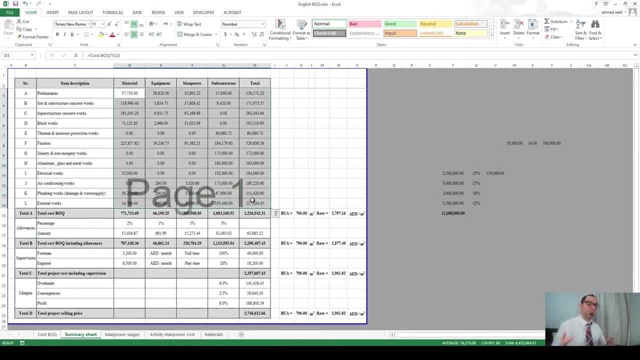 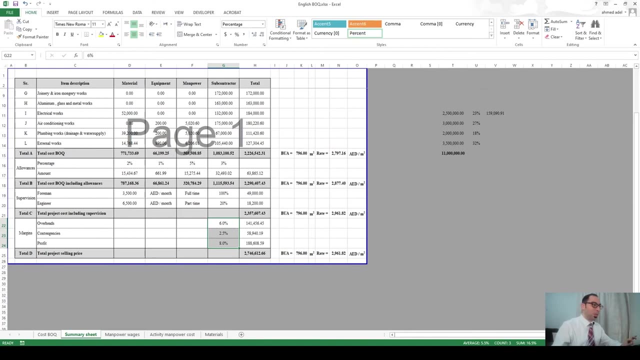 my overall margin, which is 16.5. so when this cost- okay, including the supervision, the allowances and everything else that i have priced inside, if my cost is 2.3, when i add the 16.5 percent, i will arrive a selling price. a selling. this is the price that i will give to my client. i will say to my 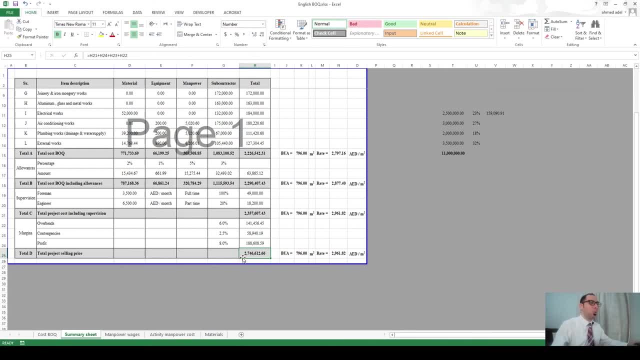 client: hi, this project will cost you 2.75 percent. so when i add the 16.5 percent, i will arrive a selling price. a selling. this is the price that i will give to my client. i will say to my client: hi, this project will cost you 2.75 percent, so when i add the 16.5 percent, i will arrive a. 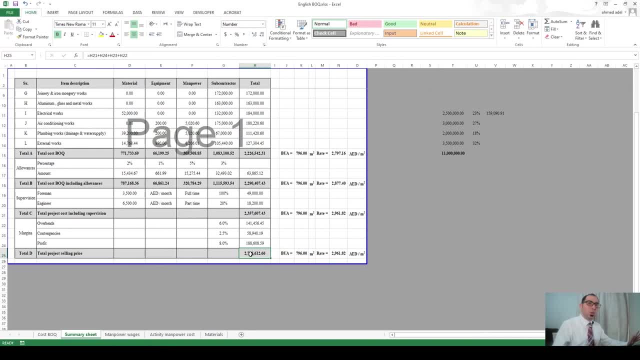 selling price, a selling, this is the price that i will give to my client. i will say to my client six and if he tries to negotiate me or if he tries to get a discount from me, the first area i will visit is these margins. if i hear, if i have like, if i have a high profit margin, maybe the market is. 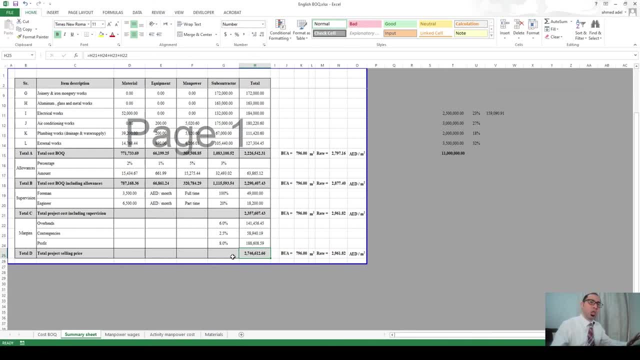 I will say to my client: hi, this project will cost you 2.74%. And if he tries to negotiate me or if he tries to get a discount from me, the first area I will visit is these margins. If I have a high profit margin, maybe the market is very competitive. 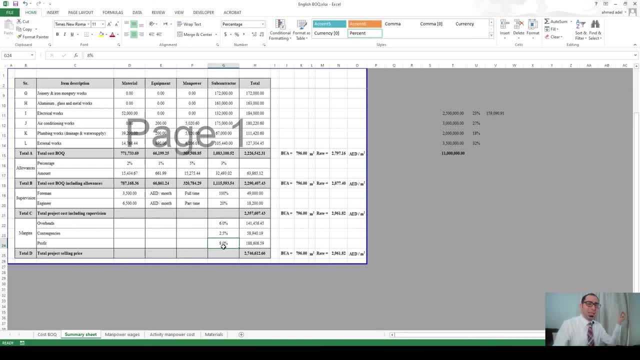 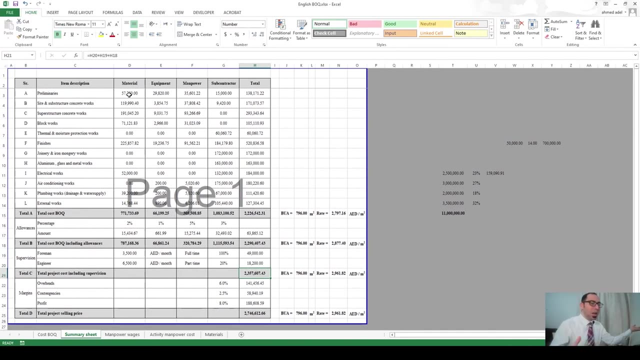 I cannot. So if I am thinking of giving him a discount, I will give a discount from these percentages. But up to here, up to the 2.3, this is, This is the calculated cost. I am assuming that the cost of this, or I estimated the cost of this project to be 2.35 million. 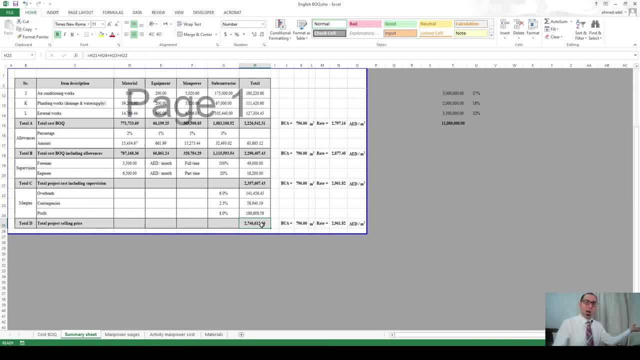 If he comes and he say: no, this 2.75 price is not accepted, I will give you only 2.35.. In that case it is up to you. You can take a project at the cost, But actually in that case you will be losing. 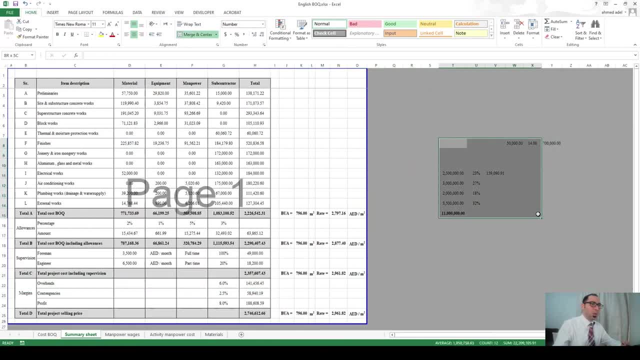 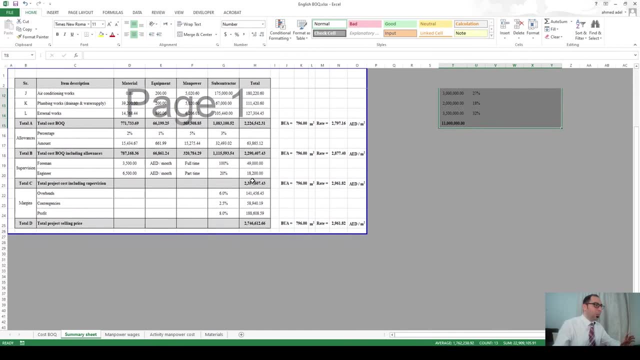 Why? Why? Because you will be running your office, As we discussed here, and your office needs from you, from this project, 160,000, almost per month, And you have not, you have not calculated that, So it cannot be done. 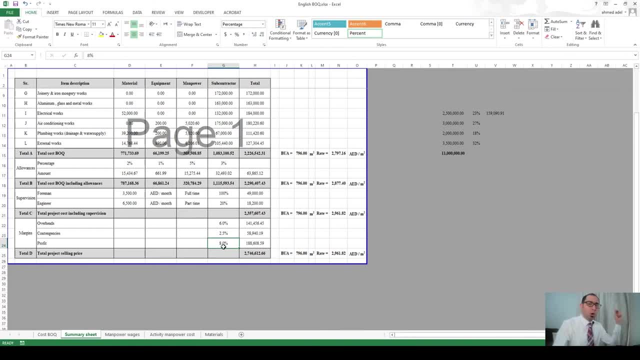 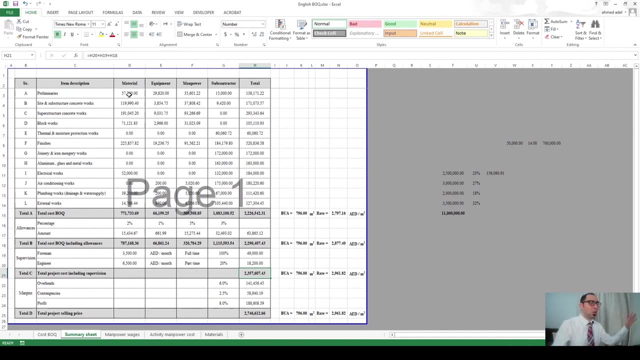 very competitive. i cannot. so if i am thinking of giving him a discount, i will give a discount from these percentages. but up to here, up to the 2.3, this is the calculated cost. i am assuming that the cost of this or i estimated the cost of this project. 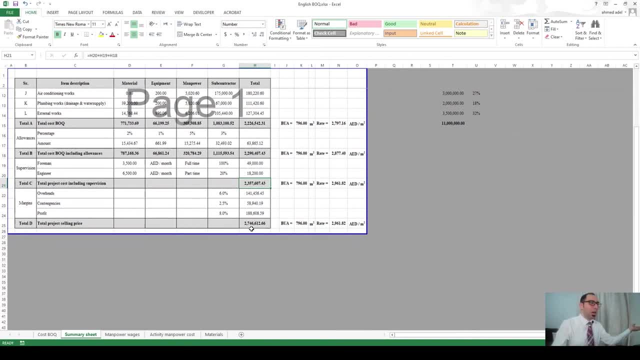 to be 2.35 million. if he comes and he say, no, this 2.75 price is not accepted, i'll give you only 2.35. in that case it is up to you. you can take a project at the cost, but actually in that case, 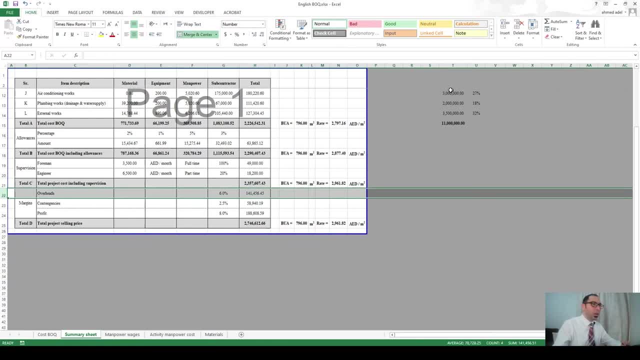 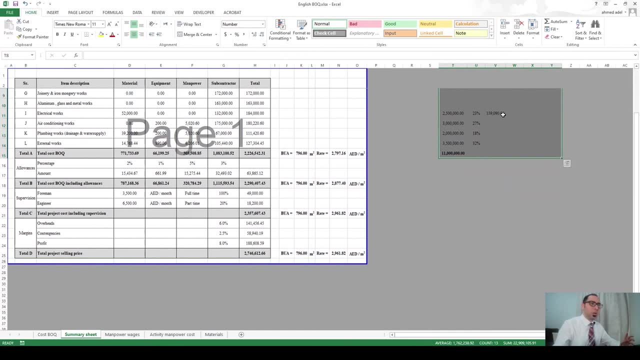 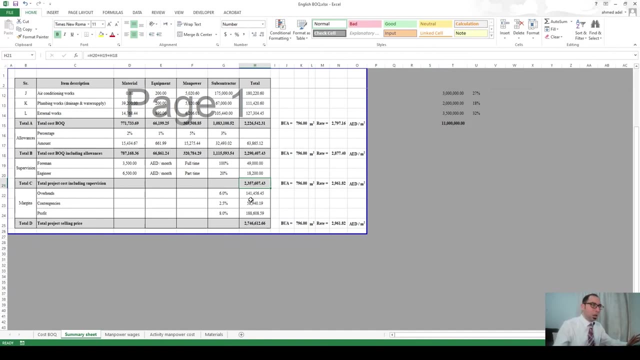 you will be losing. why? because you will be running your own project and you will be losing your own project and you will be losing your own project office, as we discussed here, and your office needs from you, from this project, 160 000 almost per month, and you have not, you have not calculated that. so it cannot be done. it cannot be done unless there 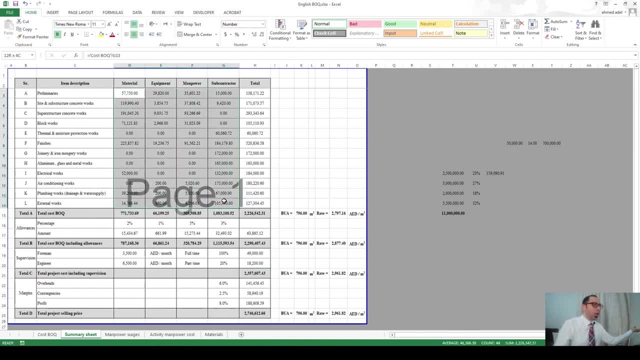 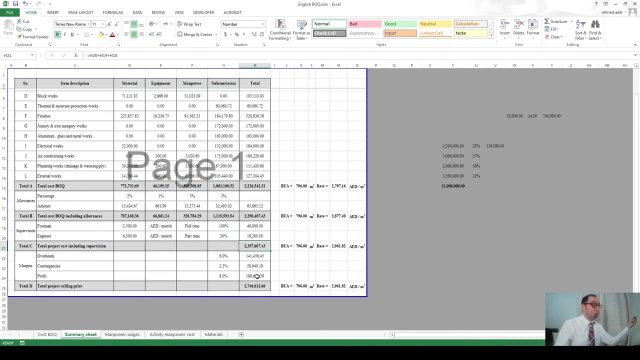 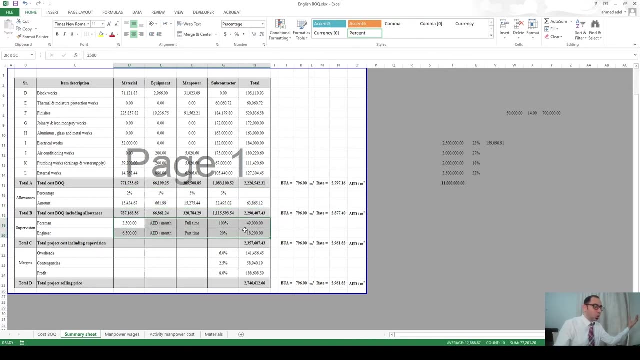 It cannot be done unless there is something like you have estimated here inside that is very high, that needs to be reduced, So it can reduce this value. But if I am sure that everything here is OK and all these things are logical, the allowances and the supervision. 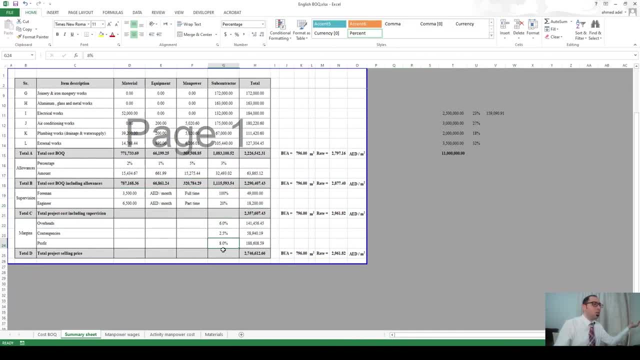 and everything- my overhead is there- then it is only the profit margin that I can reduce. instead of 8 percent, Maybe I'll put seven, maybe I'll put six and let's see. So, guys, the cost estimation is a is a is a huge world and you can understand all these concepts and all these like methodologies and all these numbers. 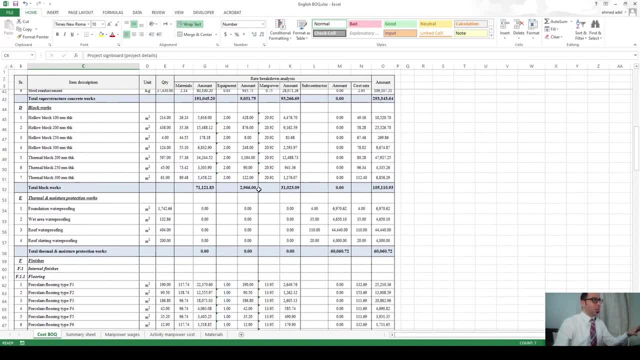 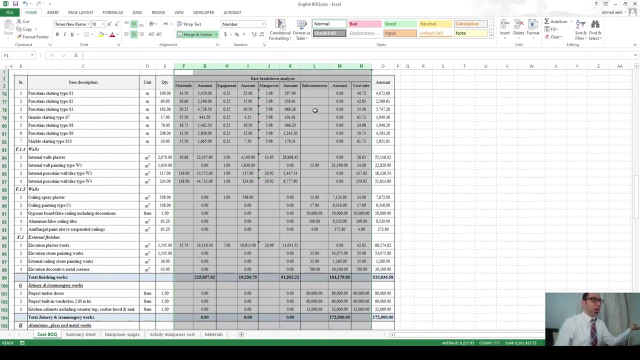 You can understand them if you practice by yourself. You need to Like, quantify one project and then start doing the rate breakdown analysis. started to start asking the vendors and the subcontractors for their prices because we live in different countries. If something is costing me here some amount, it will cost you a different amount. 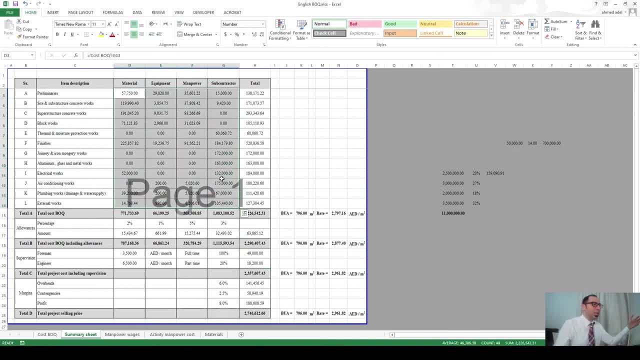 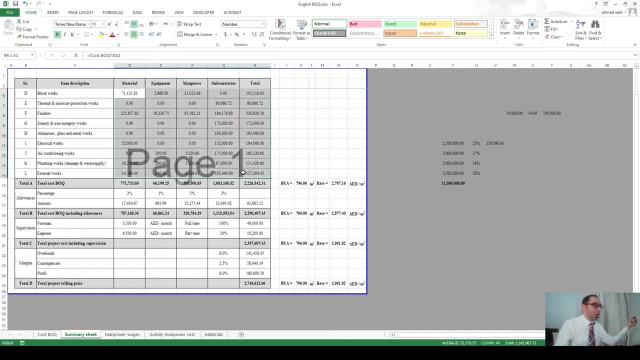 is something like you have estimated here inside. that is very high, that needs to be reduced. so it can reduce this value. but if i am sure that everything here is okay and all these things are logical, the allowances and the solutions are logical, then i will give you the cost of this project and you will be losing. 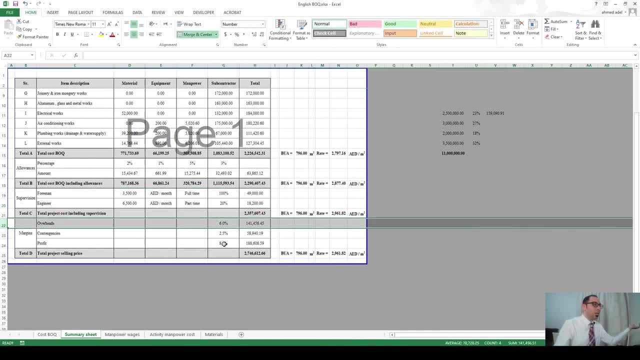 the cost of this project and you will be losing the cost of this project and you will be losing supervision and everything. my overhead is there. then it is only the profit margin that i can reduce instead of eight percent. maybe i'll put seven, maybe i'll put six and let's see. so, guys, 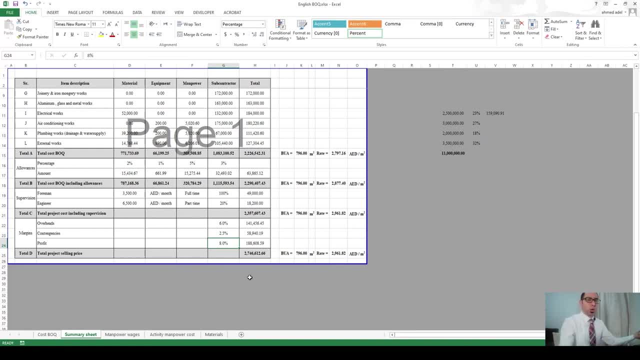 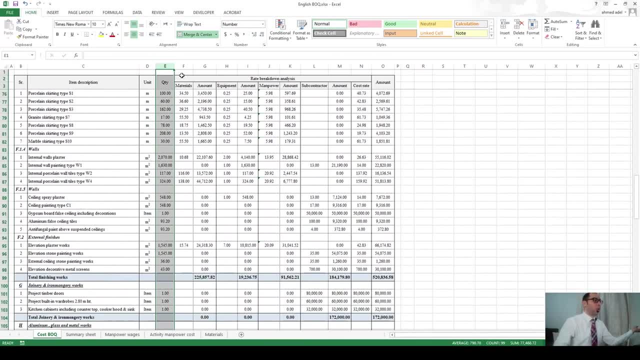 you can understand them if you practice them, if you practice them, if you practice them, you need to like quantify them. you need to like quantify them. you need to like quantify one project and then start doing the rate one project and then start doing the rate one project and then start doing the rate breakdown analysis. 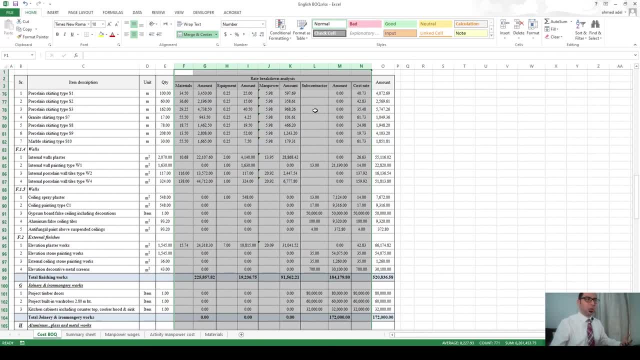 breakdown analysis. breakdown analysis started start asking the vendors and the started start asking the vendors and the started start asking the vendors and the subcontractors for their prices. because subcontractors for their prices? because subcontractors for their prices? because we live in different countries. if we live in different countries, if 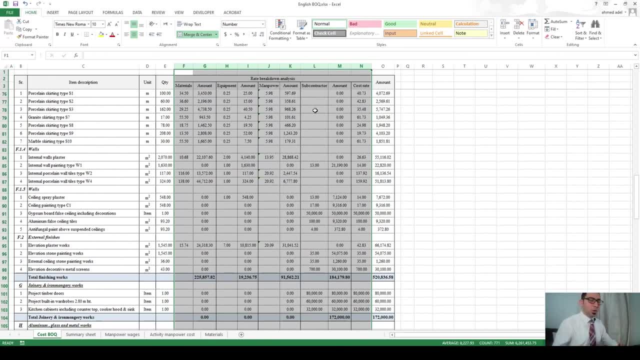 we live in different countries. if something is costing me here some amount, something is costing me here some amount, something is costing me here some amount, it will cost you a different amount, but it will cost you a different amount, but, But the concept- guys will be always same. 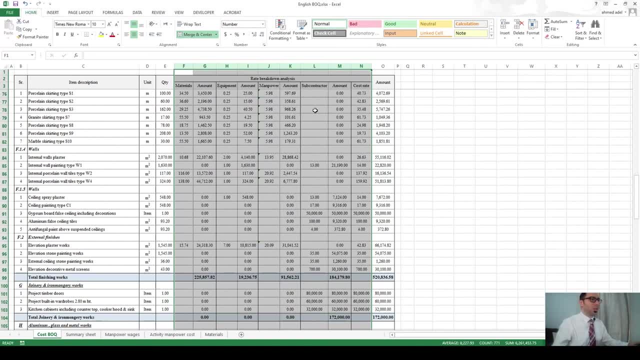 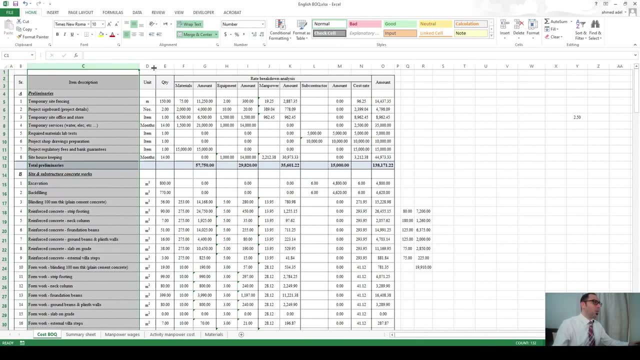 Now, I don't like promoting my courses and everything, But in the description you will find a link to our course where we have quantified a similar project. In that course we have explained in details how to get these quantities and how to prepare a BOQ from scratch. 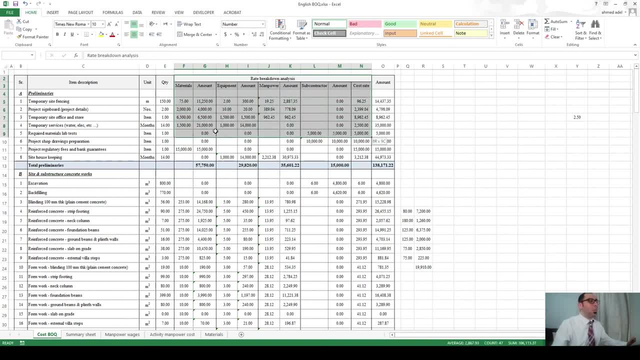 And until the moment that I am filming this video, at until this moment we have not released the cost estimation course yet, But once it is released I'll go to the description of this video and I'll update also the description And I will add the link to the cost estimation course as well. 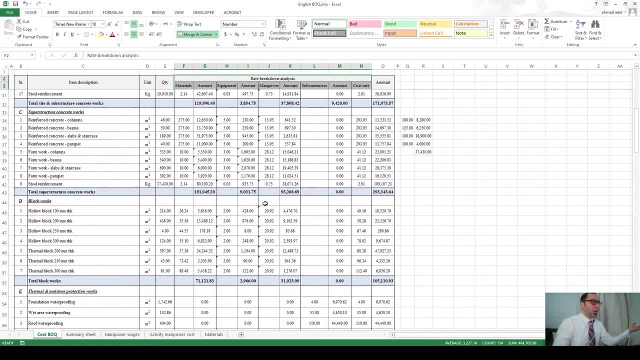 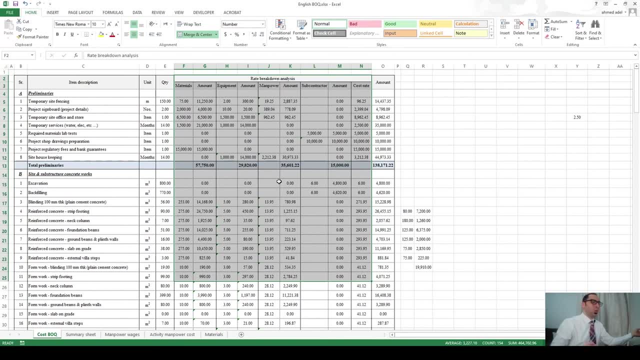 So that if you need to see in details or step by step what are all these numbers And how to do that and what to assume and what to just allow and where to allow And what all these things guys will be there in details. 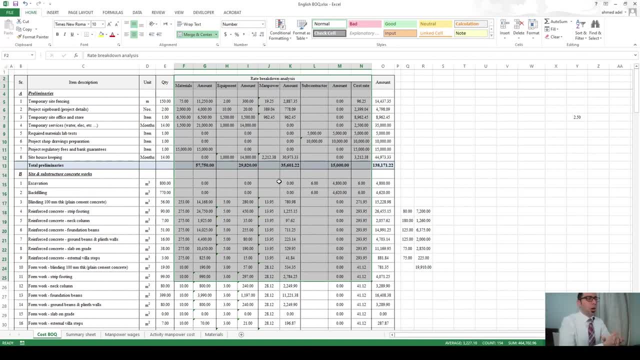 And in the end, if you guys enjoyed this video, please subscribe to notification. like, share, love, all these things. you know better now And with this guys, I'll definitely see you in the next video. 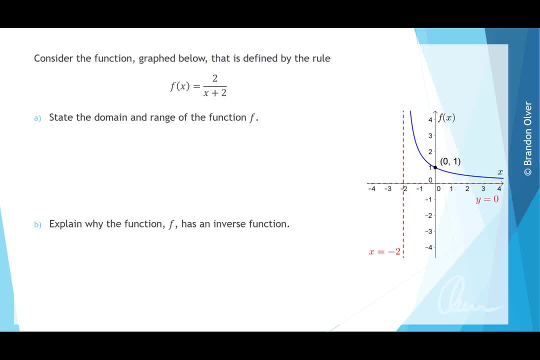 Consider the function graph below. that is defined by the rule f of x equals 2 divided by x plus 2.. For part a, we want to state the domain and range for the function f. So to do this, we're going to set up a table to hold our information. 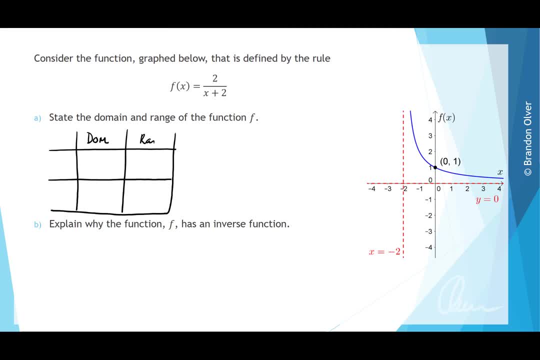 So in this column we're going to put the domain and in this column we're going to put the range. For this row we're going to consider the function f and in this row we're going to consider f- inverse. So for f the domain goes from negative 2 to infinity. 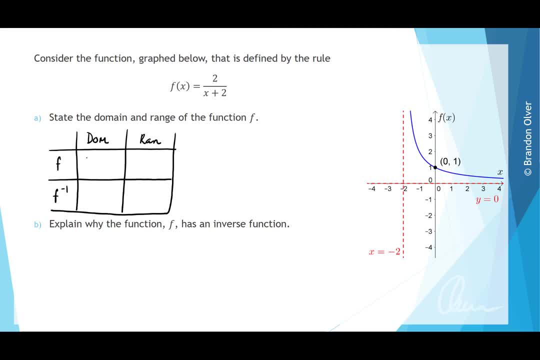 They are all the x values that are allowed inside this function. So it's from negative 2 to infinity. in interval notation, where the 2 is excluded and the infinity is excluded with a round bracket, The range you can observe goes from y equals 0, not included, up to infinity. 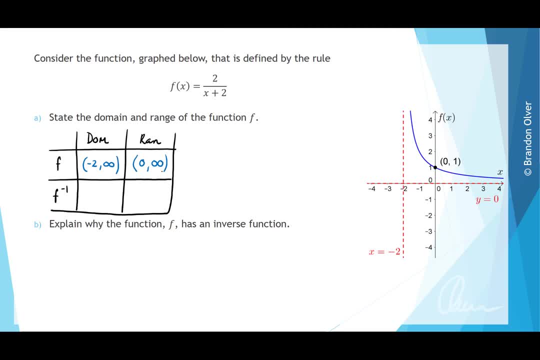 So we're going to have 0 not included to infinity, with a round bracket. Now, even though it doesn't ask for it, we've drawn in two extra cells To contain the information for the domain and range of the inverse function, And these will just come in handy later on. 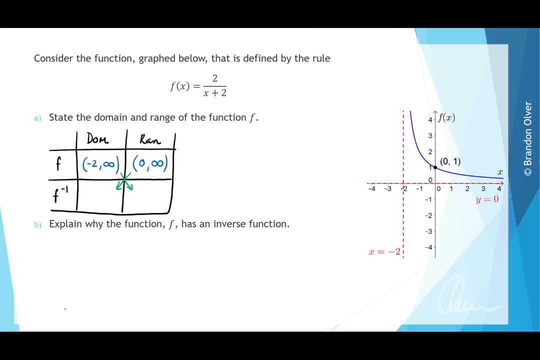 So we swap the domains and ranges for inverse functions. So we will eventually discover that the domain of f- inverse is 0 to infinity And that the range is from negative 2 to infinity. For part b we want to explain why the function f has an inverse function.